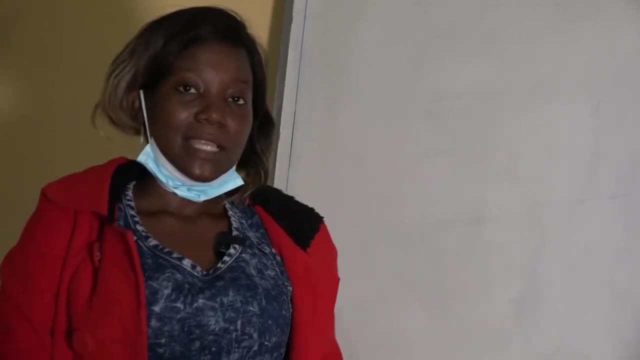 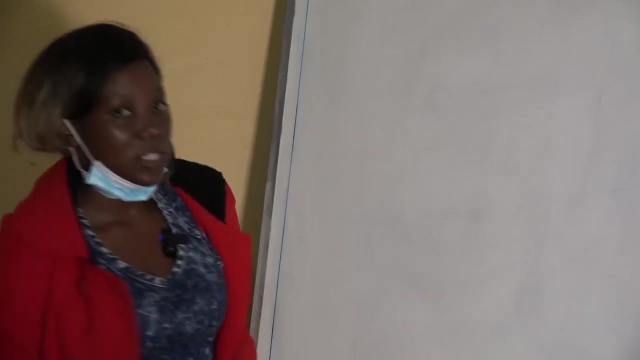 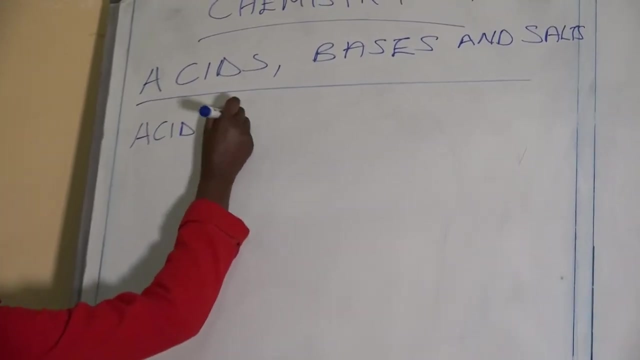 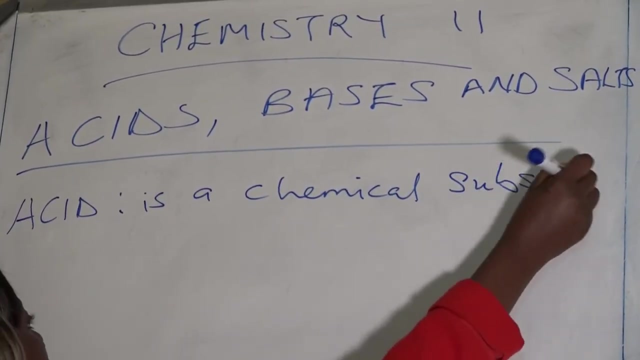 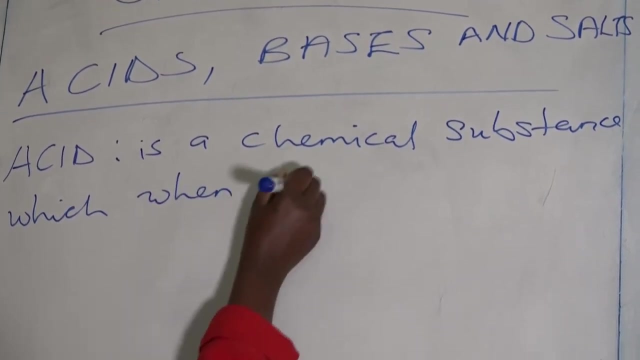 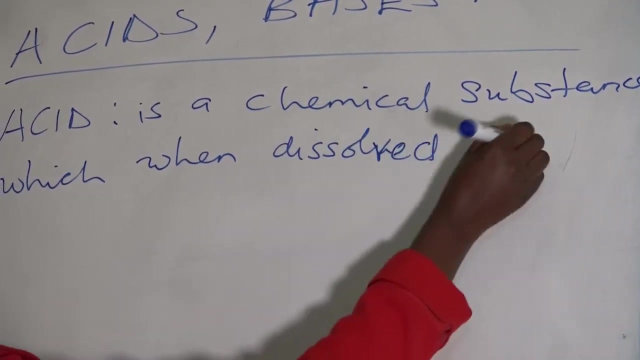 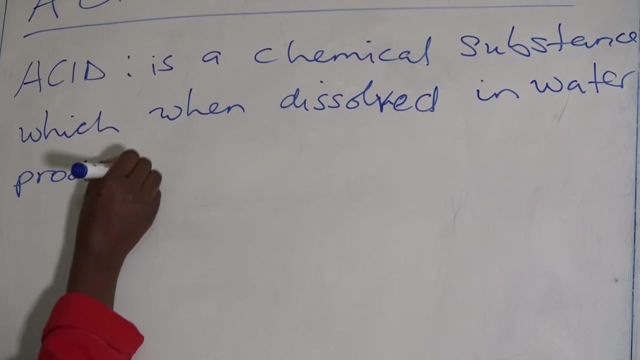 acids. So an acid is a chemical substance which, when dissolved in water, produces hydrogen ions as the only positively charged ions. I repeat: an acid is a chemical substance which, when dissolved in water, produces hydrogen ions as the only positively charged ions. 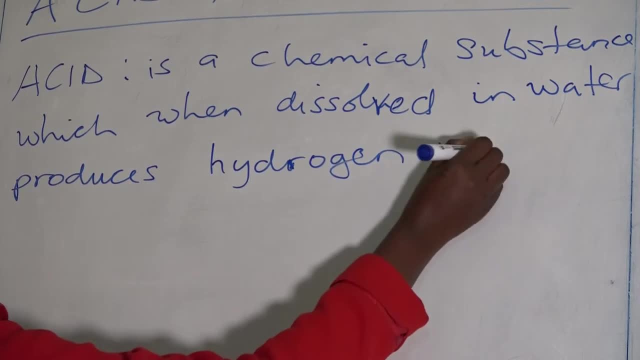 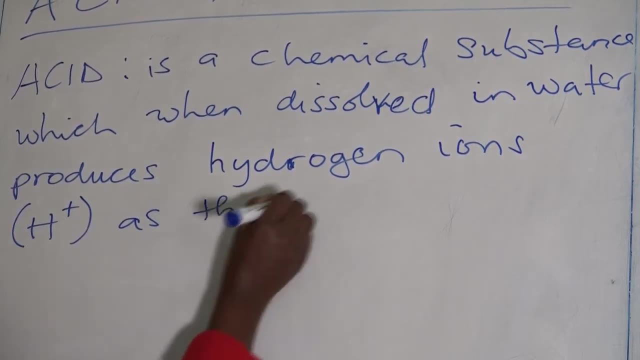 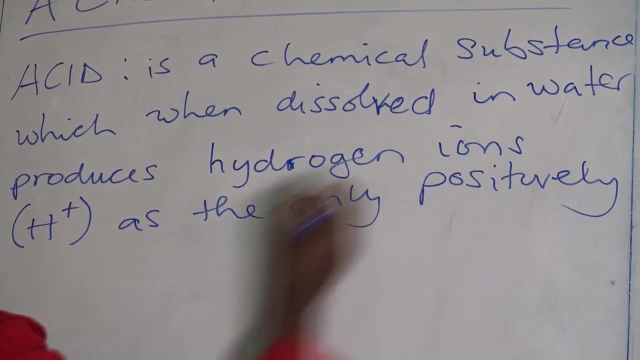 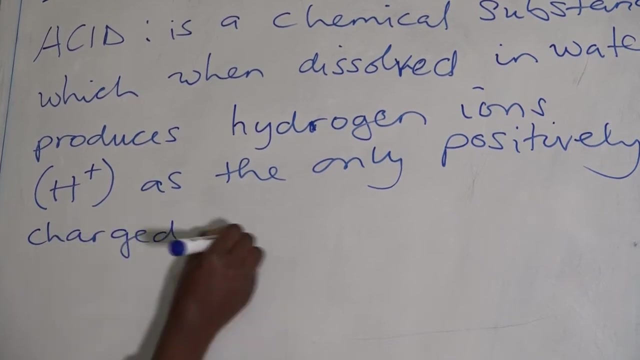 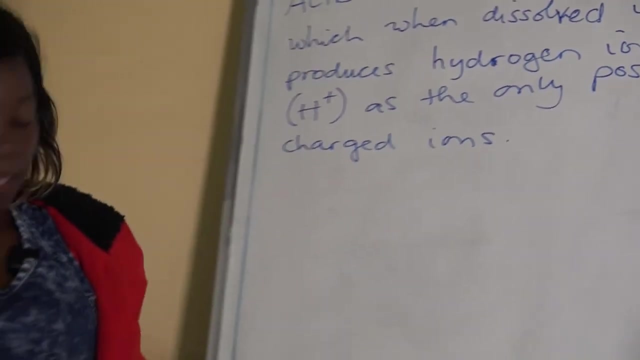 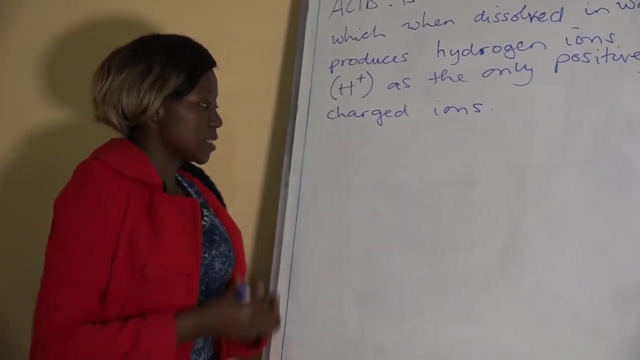 So an acid is a chemical substance which, when dissolved in water, produces hydrogen ions as the only positively charged ions. So an acid is a chemical substance which, when dissolved in water, produces hydrogen ions as the only positively charged ions. So an acid is a chemical substance which, when dissolved in water, produces hydrogen ions as the only positively charged ions. 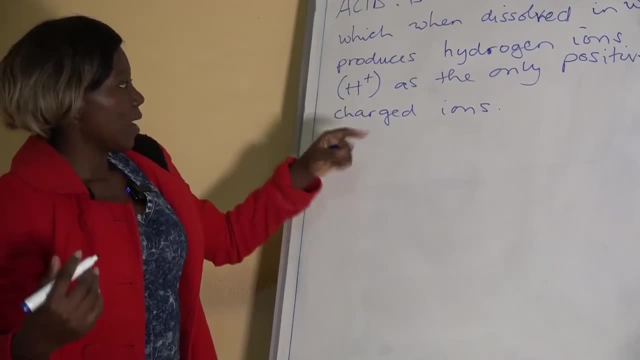 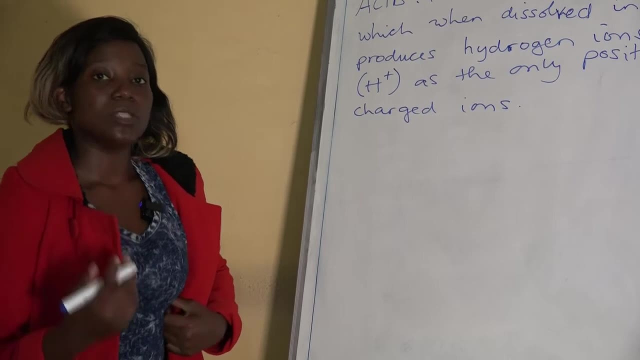 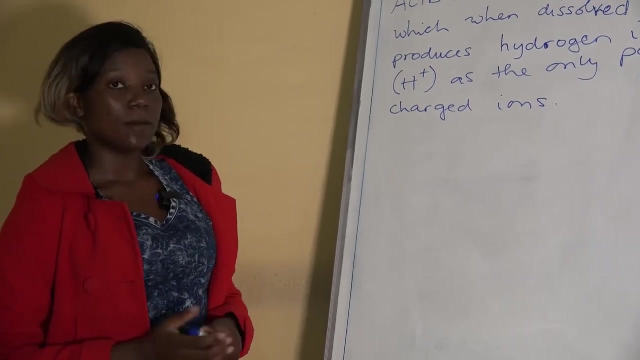 Meaning this hydrogen ion, when this particular substance dissolves in water, will be the only product in a chemical reaction that will be positively charged. It will be the only product to be positively charged and in this case it is a hydrogen ion. 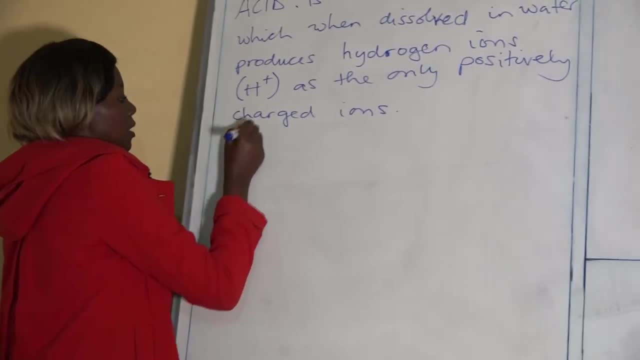 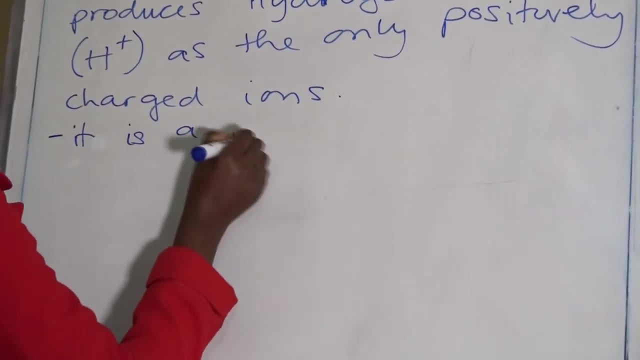 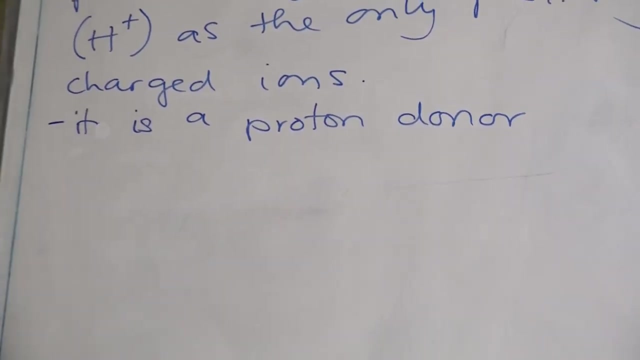 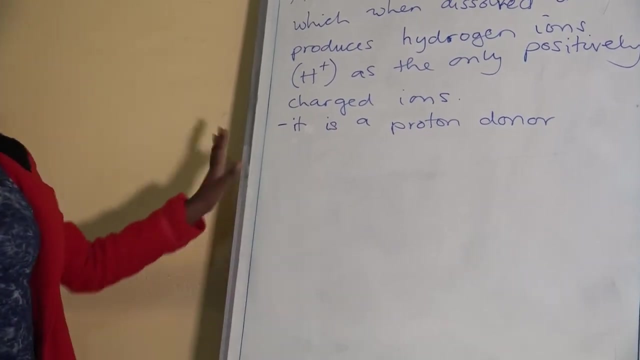 Okay, Okay, Okay, Okay. Okay said to be a proton donor. what do you understand by the term proton donor? because it is producing hydrogen ions as the only positively charged ions. we expect that it is going to donate this proton from the positively charged. 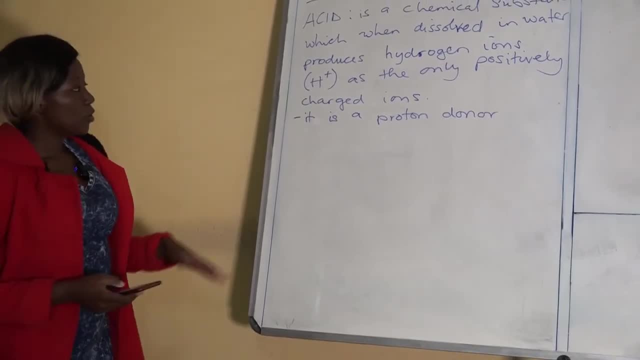 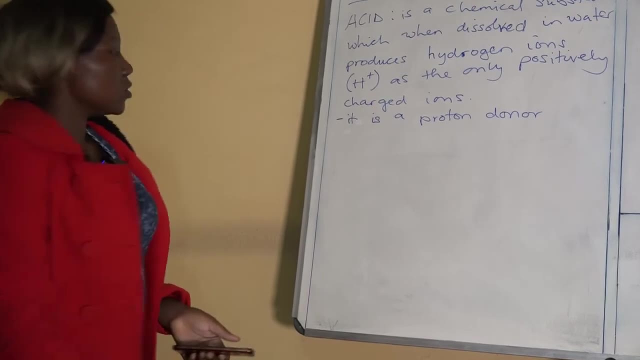 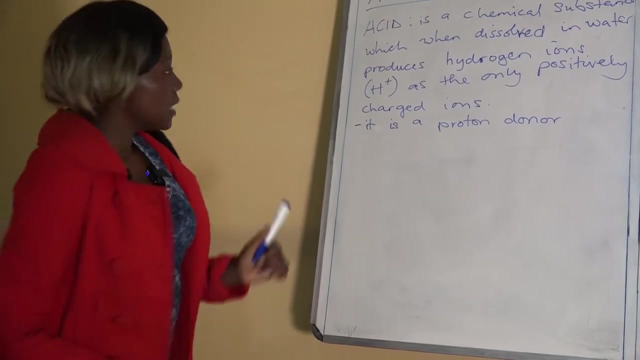 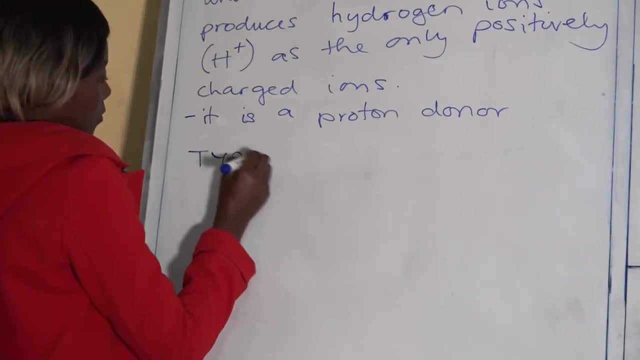 hydrogen ion to be the only proton in the products of the reaction and therefore it is said to be a proton donor. an acid is also said to be a proton donor. now, acids are of two types. we have two types of acids. these are number one, two types of acids. number one. we have mineral acids, which are, of course, formed from naturally occurring mineral elements. these are formed from naturally occurring mineral elements because you have seen that they are mineral, and they are also formed from naturally occurring mineral elements because you have seen that they are mineral acids. obviously they are formed. 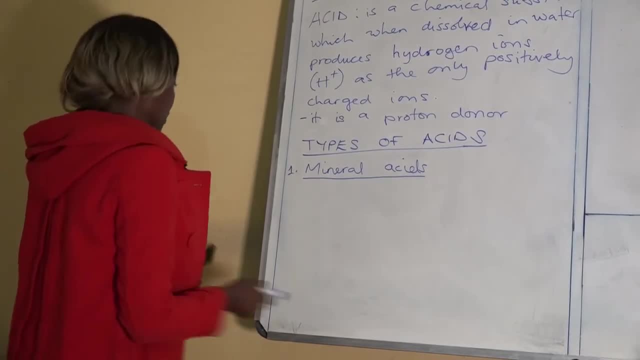 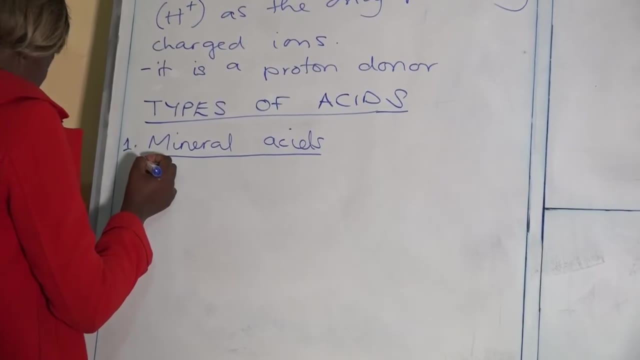 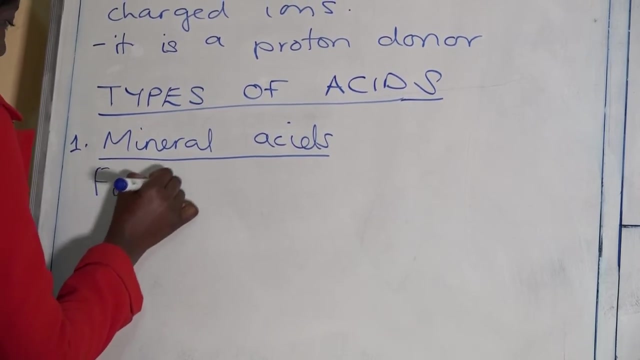 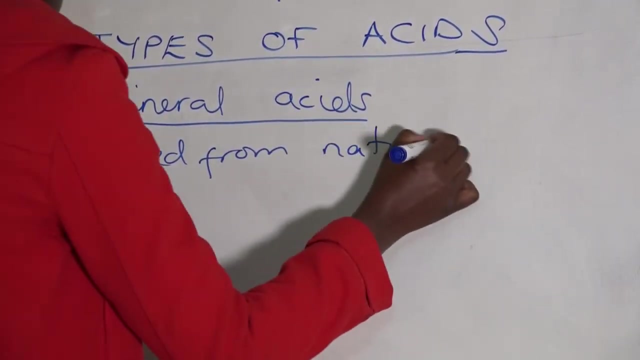 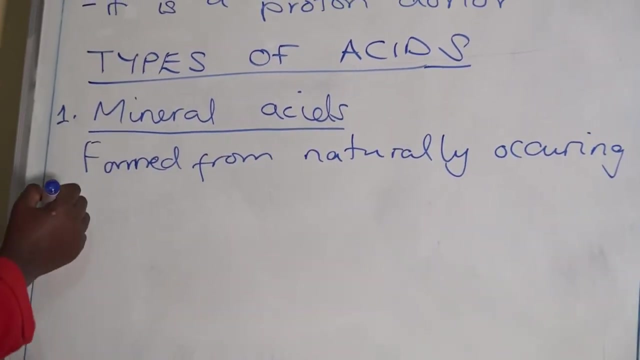 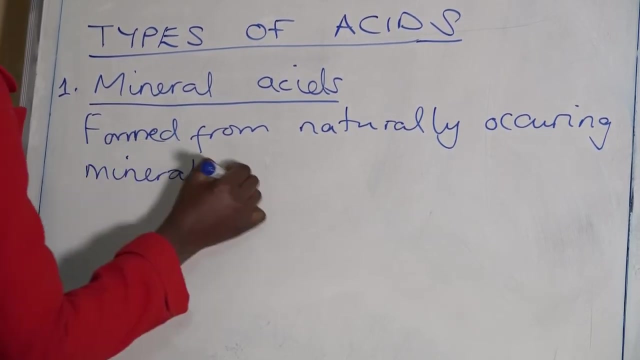 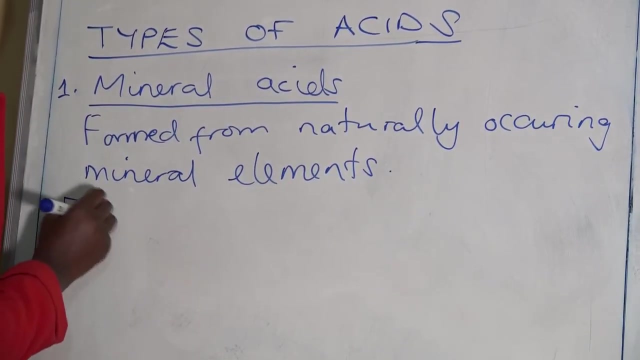 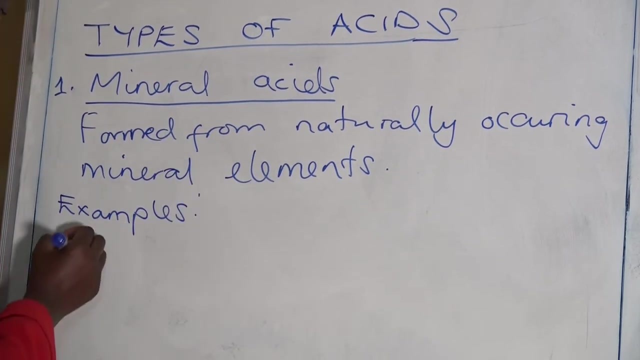 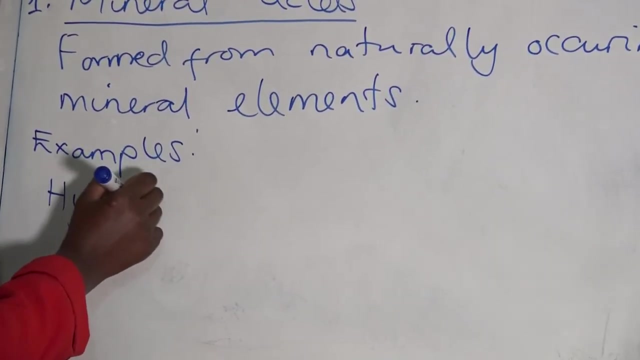 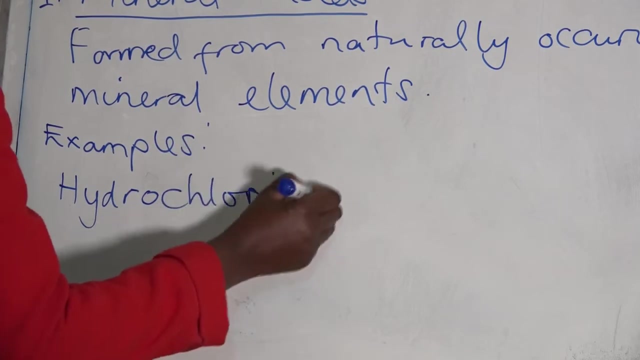 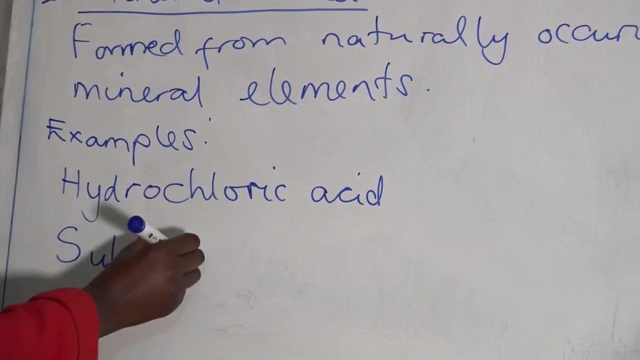 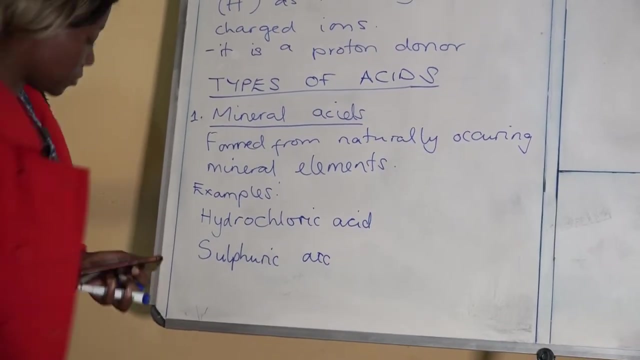 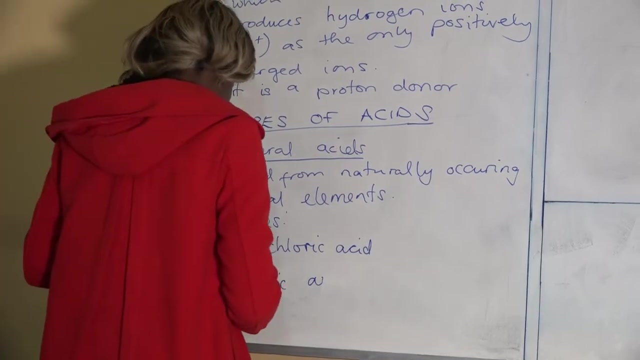 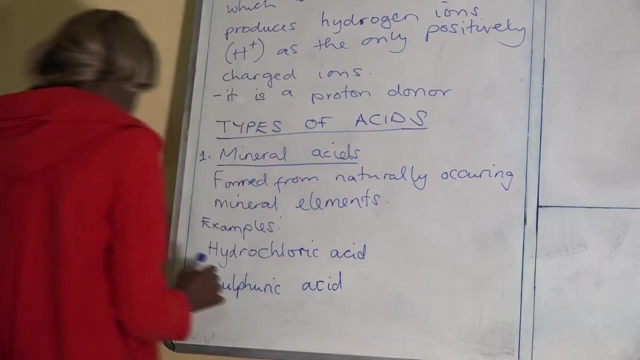 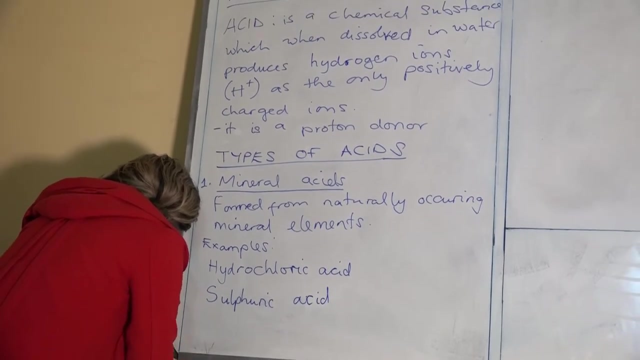 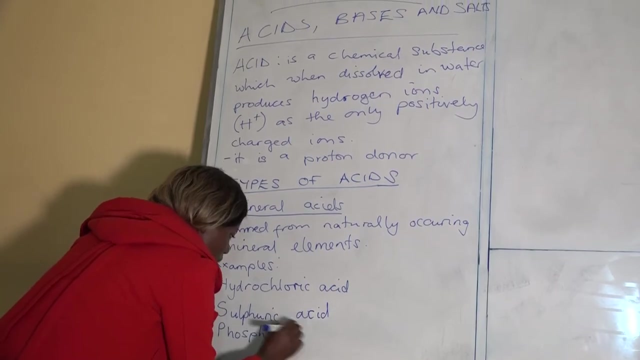 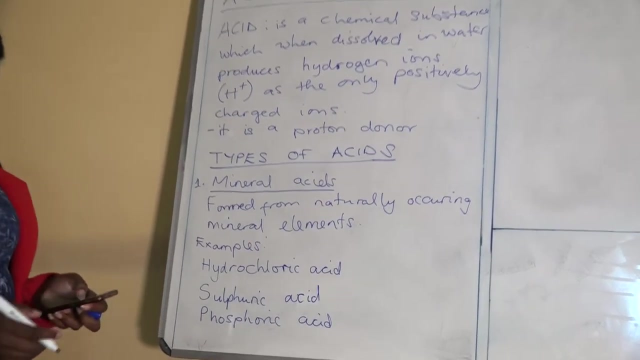 from naturally occurring mineral elements. formed from naturally occurring mineral elements. examples are hydrochloric acid, hydrochloric acid, and, and, and and Sulfuric acid, Phosphoric acid, Etc. So we have hydrochloric acid, Sulfuric acid, Phosphoric acid. 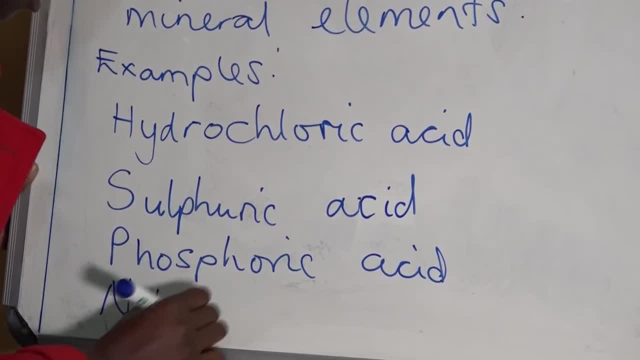 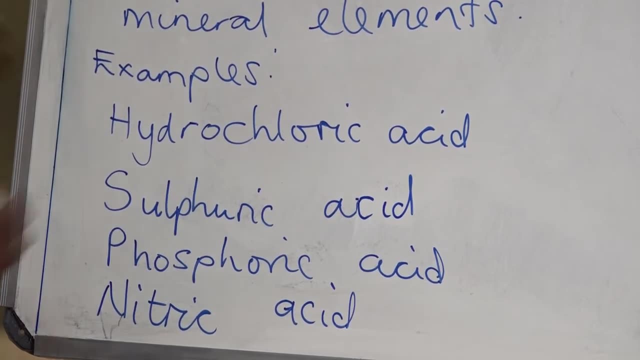 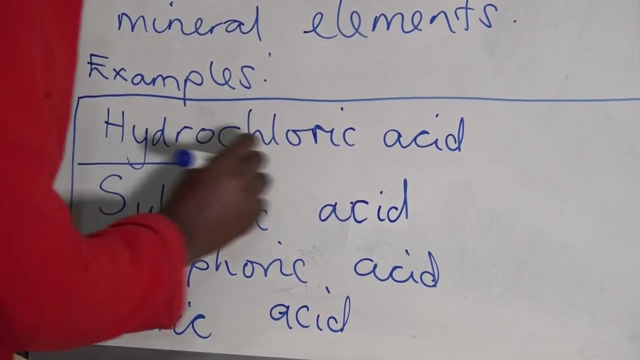 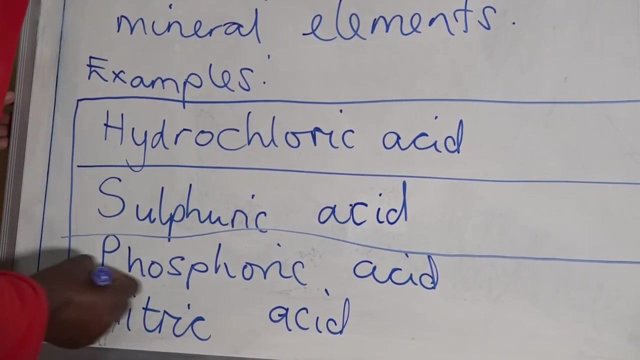 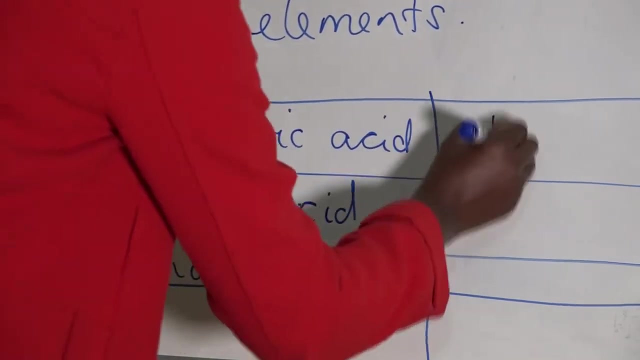 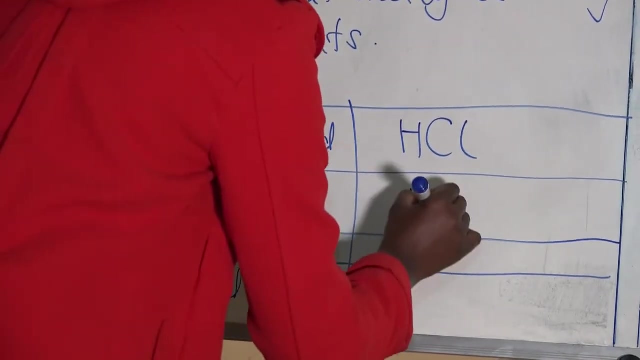 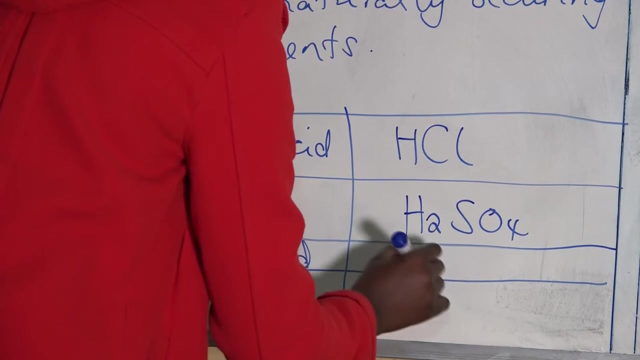 Sulfuric acid, Nitric acid, Etc. So now these, I'll give you symbols For the examples. Okay, Hydrochloric acid, Hydrochloric acid. Hydrochloric acid Is HCl. Okay, Sulfuric acid: H2, SO4, Nitric acid. 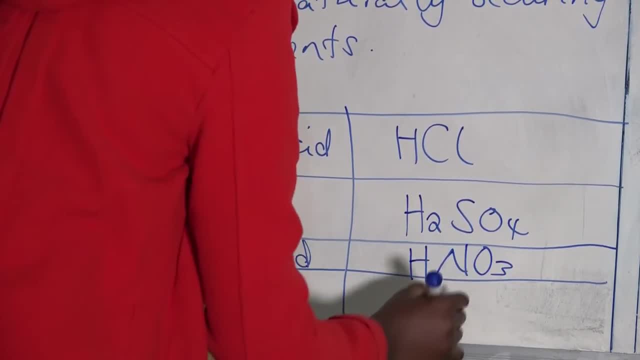 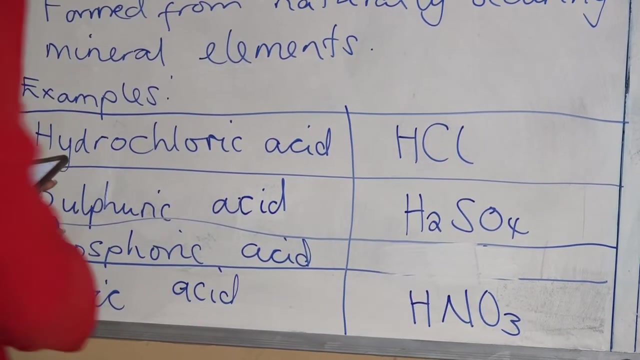 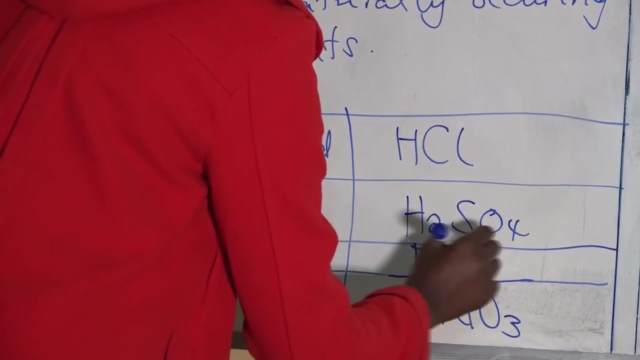 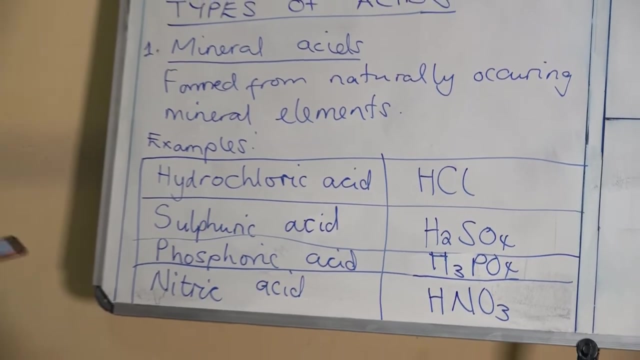 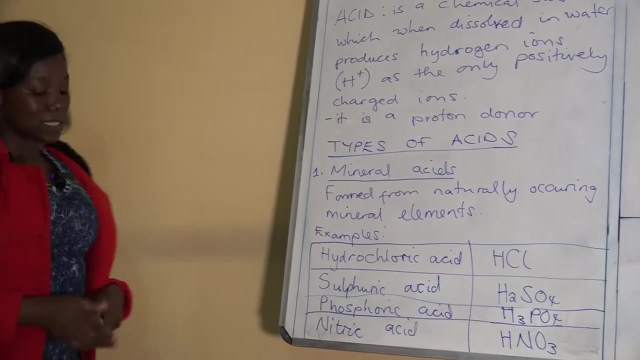 HNO3 And, Sorry, Phosphoric acid. HNO3 And Phosphoric acid. Phosphoric acid Is H3, PO4. Okay, These are examples Of mineral acids. Mineral acids: They are acids That are prepared From naturally Occurring mineral elements. These are types of acids. 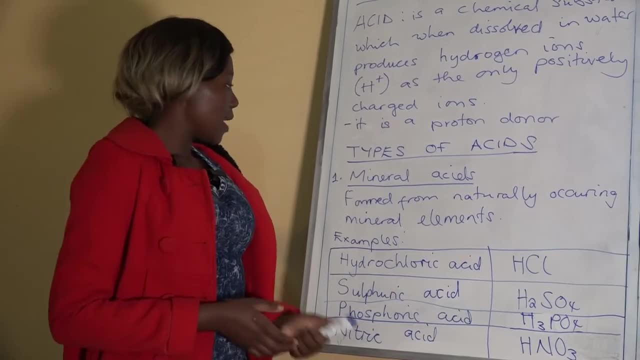 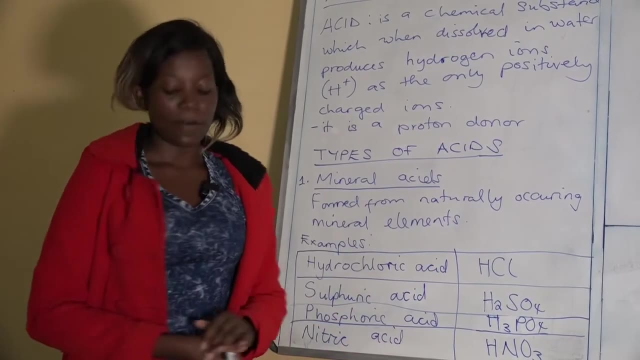 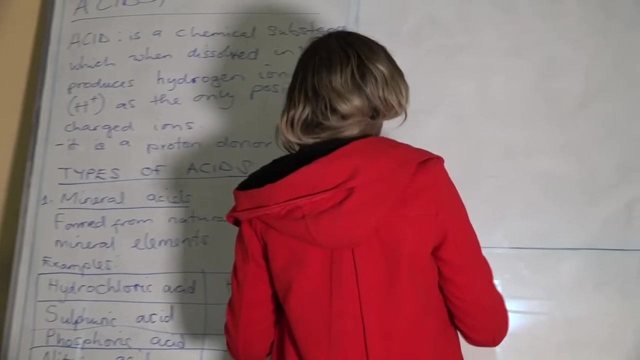 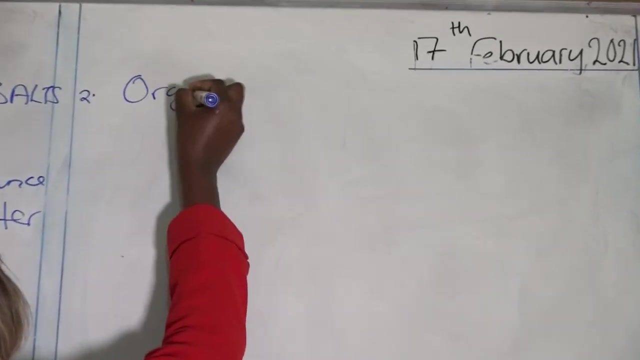 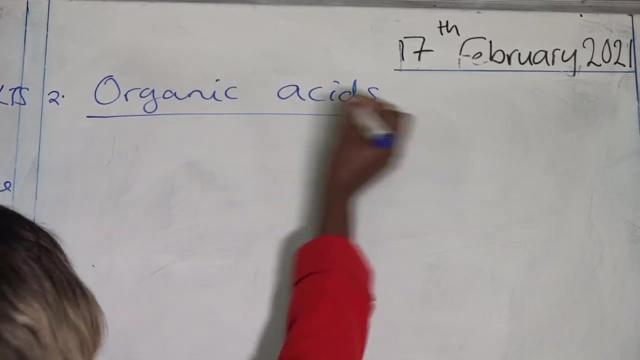 I said, acids Can be classified Into two. Number one: We have looked at Mineral acids, Which are acids That occur, That are formed From naturally Occurring elements. The second type Of acids Are organic acids. The second type Of acids Are organic acids. Number two: Organic acids. These are formed. 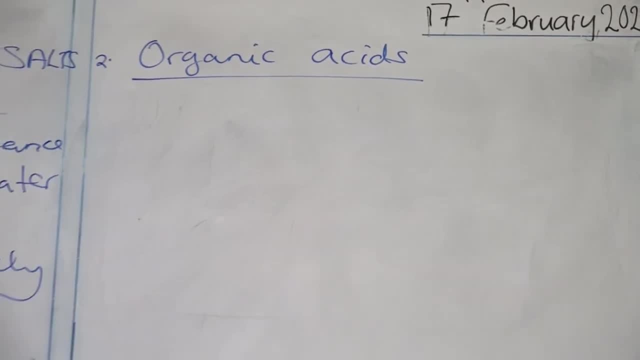 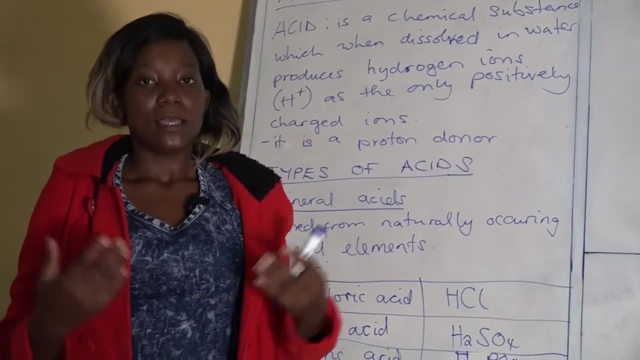 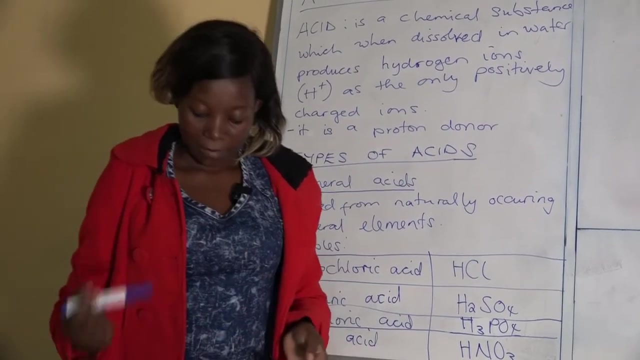 From Phosphoric acid Plants, And These are formed From plants And naturally Occurring Living organism Matter. These are formed From Matter Such as That of living organisms. They are formed From Natural Organisms Such as Plants. These are formed From Natural Matter Such as Plants. Okay, They are formed. 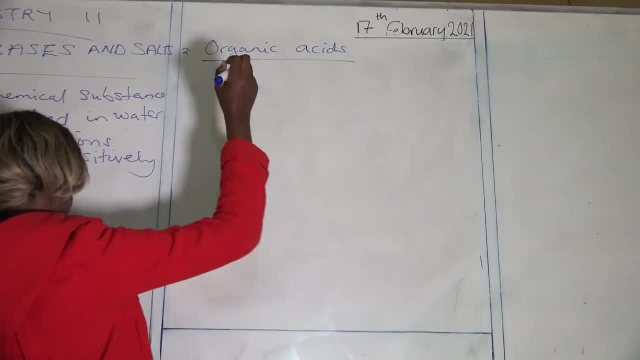 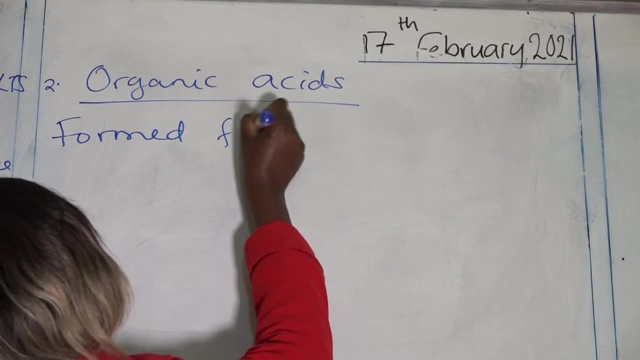 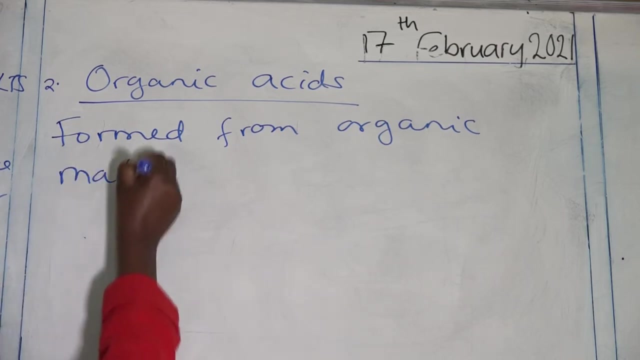 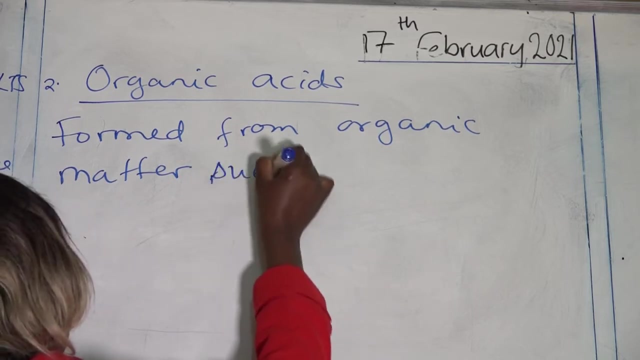 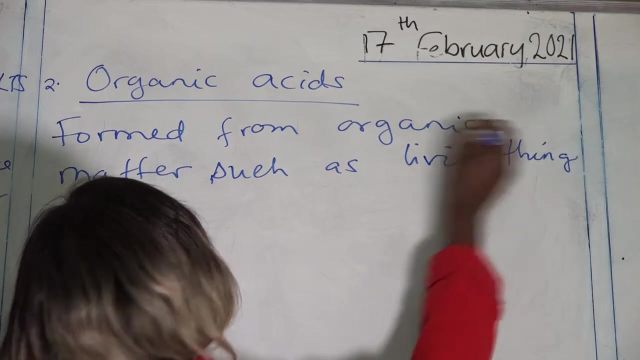 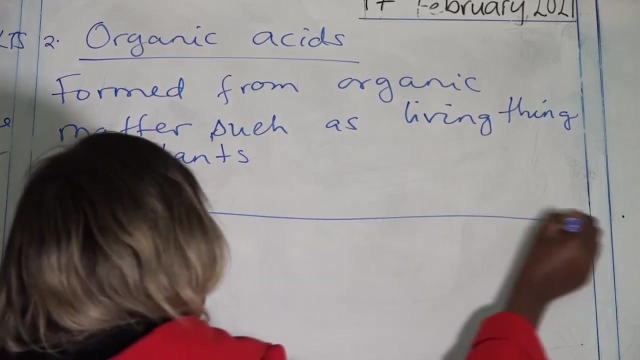 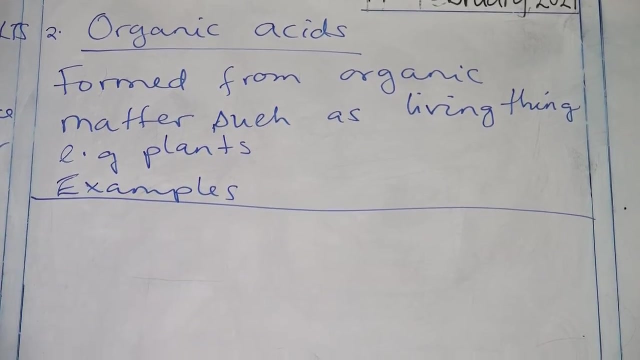 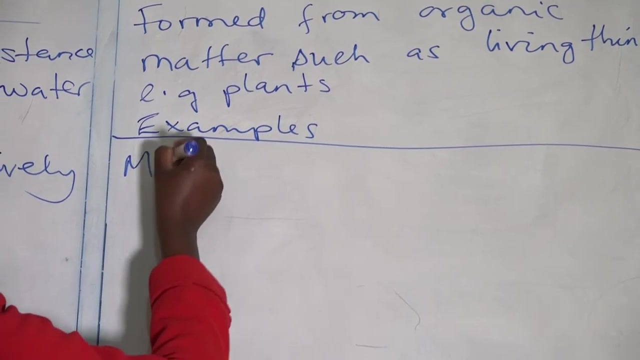 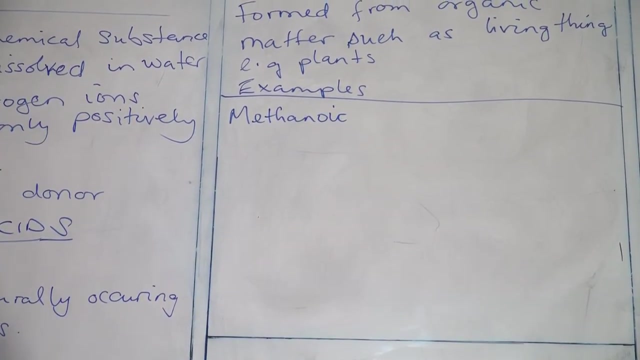 From natural matter, Naturally Occurring Organic matter. These are formed From organic matter, Okay, Such as Plants, Eg Plants, Okay, and Examples of These, Examples Of Mineral Examples, Sorry, Of Organic acids. We have Meta Methanoic Acid, Okay, Ethanoic Acid Propanoic. Acid, Methanoic Acid, Propanoic Acid, Carbonic Acid, Methanoic Acid, Methanoic Acid. Those are Examples of Naturally Occurring Living matter Acid Such as That we That we are Calling Organic Acid. Sorry, These are Examples of Organic Acids Which we Said Are formed From Naturally Occurring Organic Matter. Okay. Methanoic Acid, Ethanoic Acid, Methanoic Acid, Propanoic Acid And Butanoic Acid. Symbols: H, C O O, H, H, C, H, Three C, Two, H, Five C O O, H And. 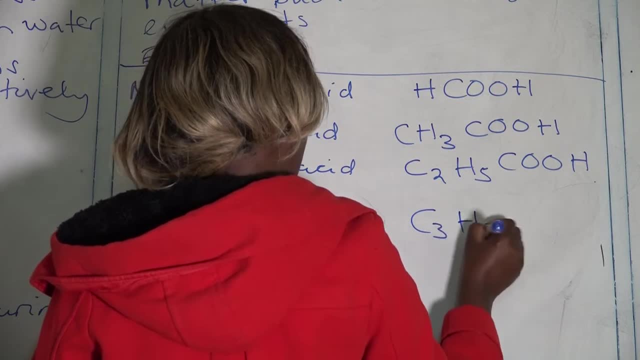 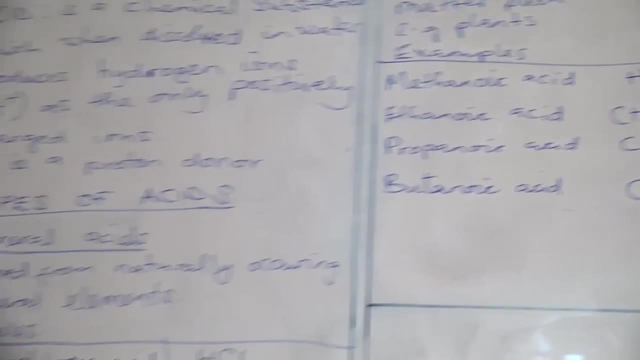 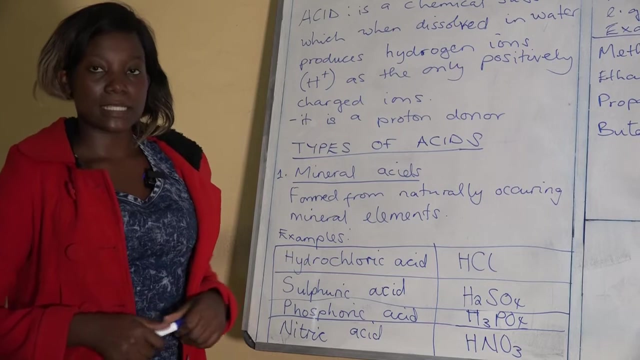 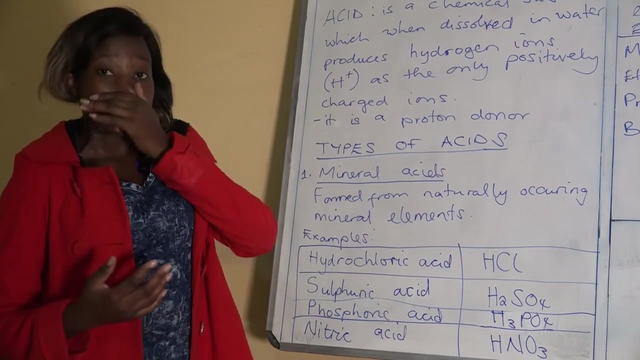 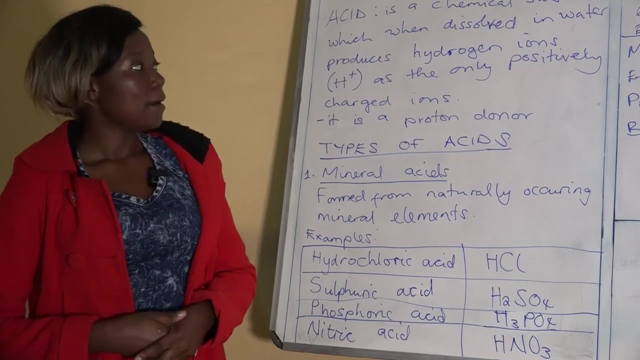 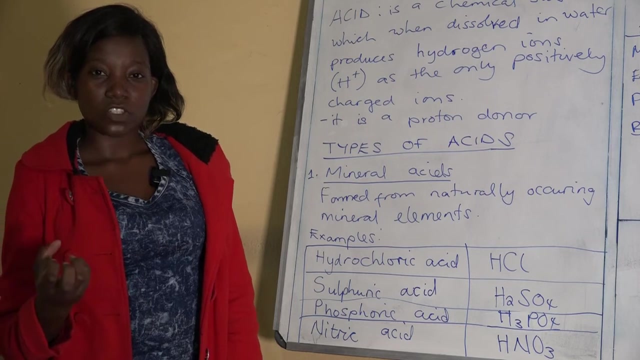 C, Three, H, Seven C O O H. So For Now, All You Need To Know Is That Mineral- Sorry- Organic Matter, It Is Living Matter, It Is Matter From Living Things And EG. We Have Plants. Okay, Decaying Matter From Plants Is Organic Matter And These Acids Are Formed. 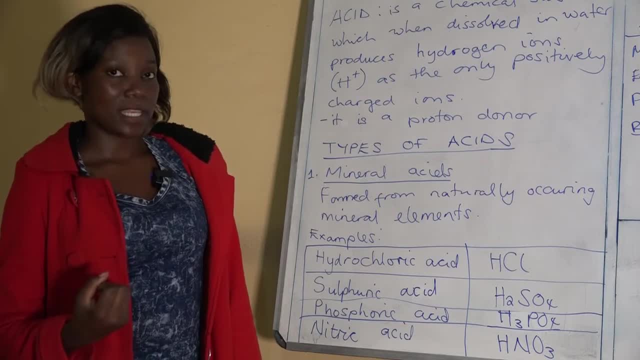 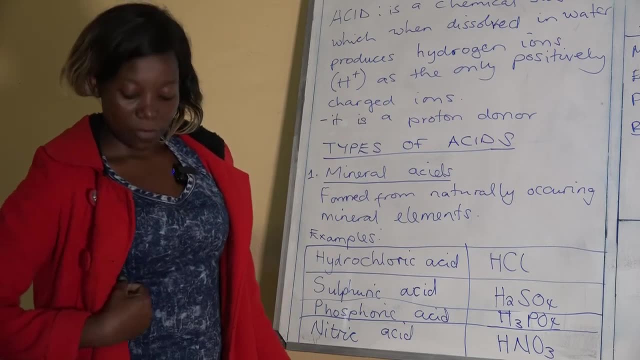 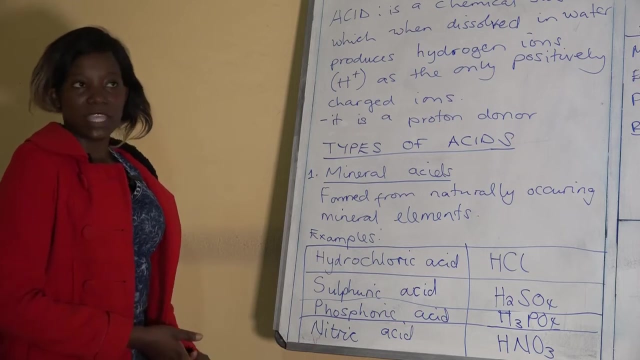 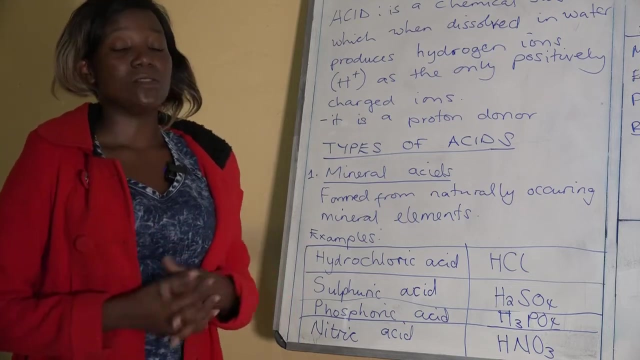 From Such Kind Of Matter, So The Acid You Find In Orange Or Lemon Acid. That Is The Difference. The Acid We Get From Metals Is Mineral Acid. The Acid We Get From Living Matter Such As Plants, Of Course Lemons, We Know There Is Acid In Lemon. There Is Acid. In Orange. Most Of Our Fruits And Some Bitter Vegetables Have Quantities Of Acid In Them And That Is Two Types And We Have Said These Are Mineral And Organic Acids, That Two Types Of Acid: Mineral Acids And Organic Acids. So Let's Move. 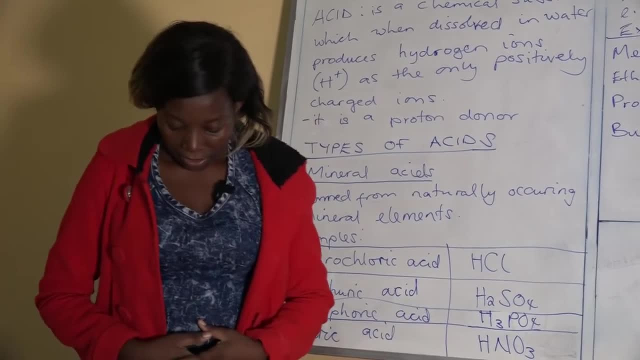 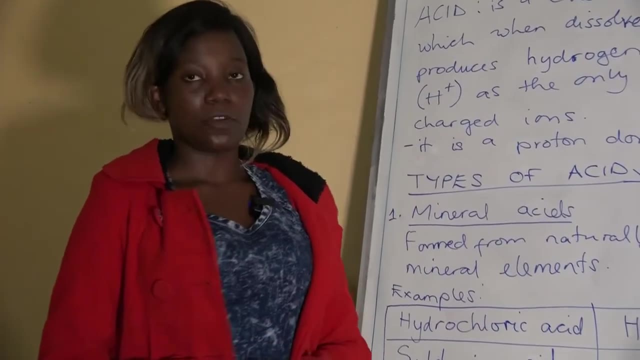 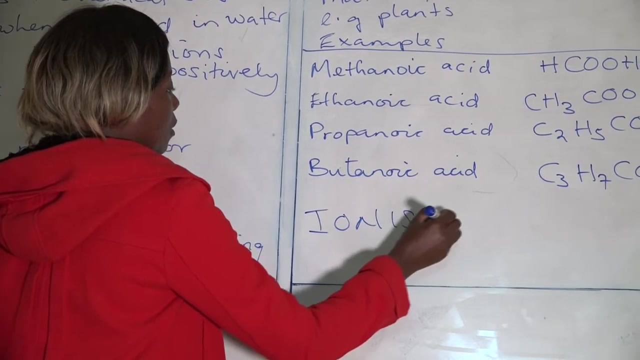 On And Look At Ionization Of Acids. What Is Ionization Of Acids? What Is Ionization Of Acids To Be Ionized? Ionization Is Simply The Forming Of Ions. Ionization Is Simply The Forming Of Ions. This Simply Means The Formation. 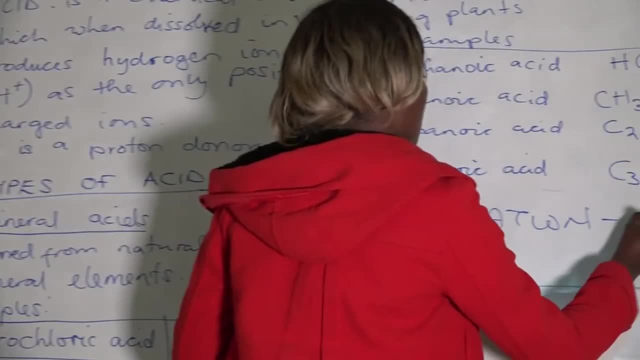 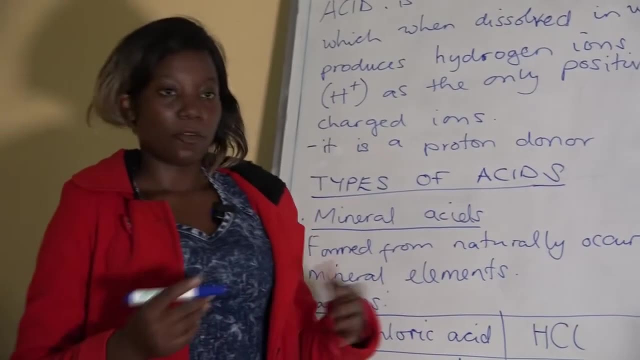 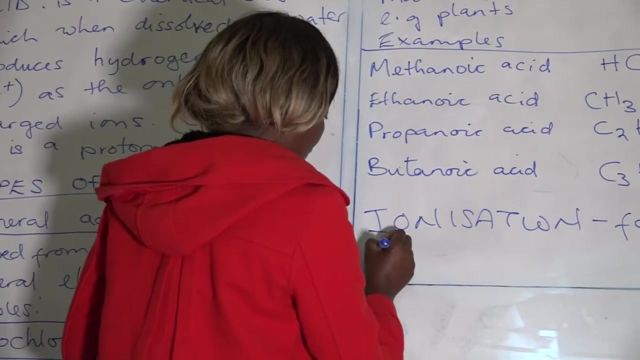 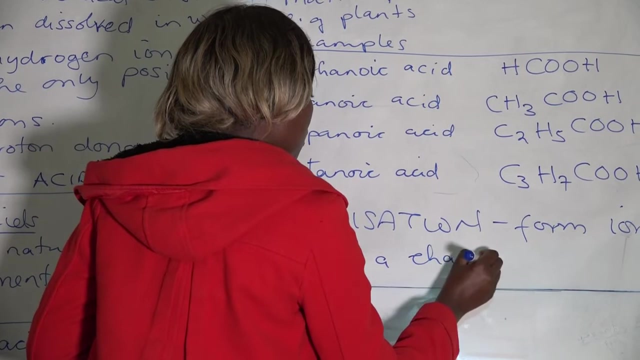 Of Ions. We Are Forming Ions. This Is To Form Ions, And I Am Sure From Grade 10 You Learned That An Ion Is A Charged Particle Or Atom. An Ion Is A Charged Atom. Okay, So If An Ion Is A Charged, 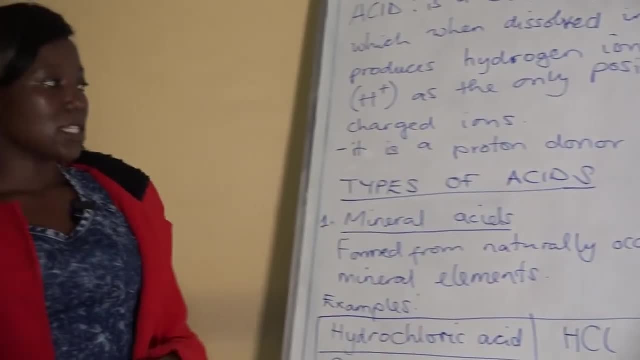 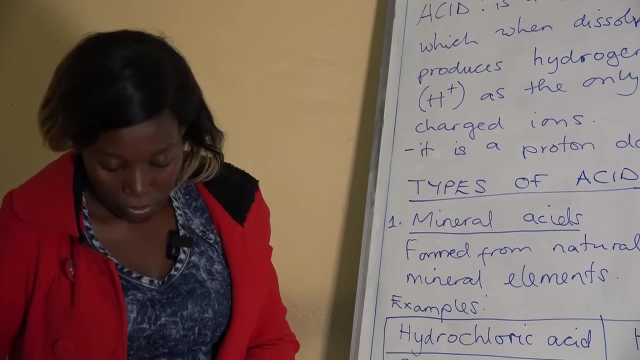 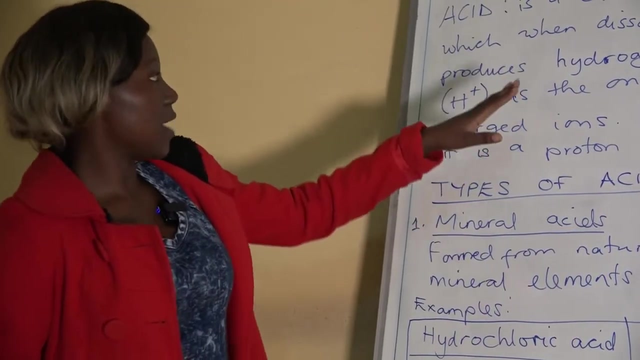 Atom In The Ionization Of Gases. We Are Simply Charging Atoms Or We Are Simply Forming Charged Atoms. Okay, So When Acids Dissolve In Water, They Produce Hydrogen Ions. That From The Definition We Have Given Here. When The Ions Are The Only Positively Charged Ions. They Produce Hydrogen Ions As The Only Positively Charged Ion. So In Ionization Of Gases We Are Simply Separating The Hydrogen, Making It The Only Positively Charged Ion, From Our 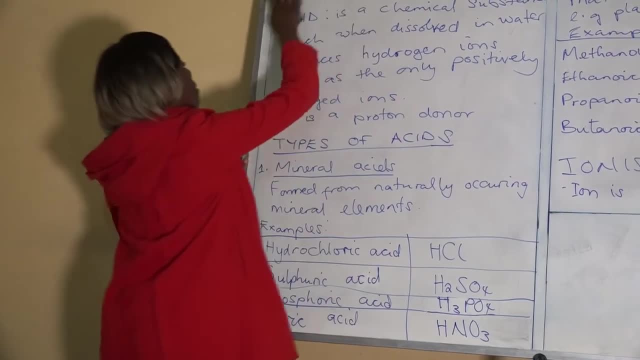 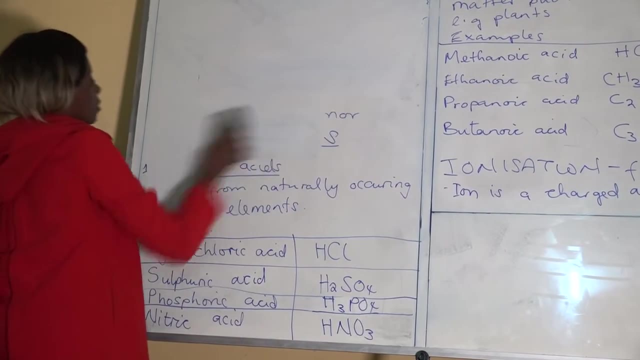 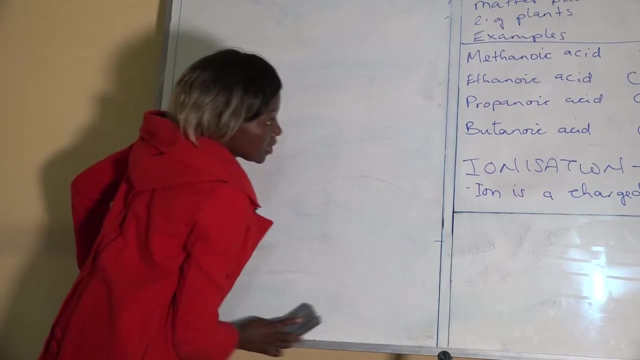 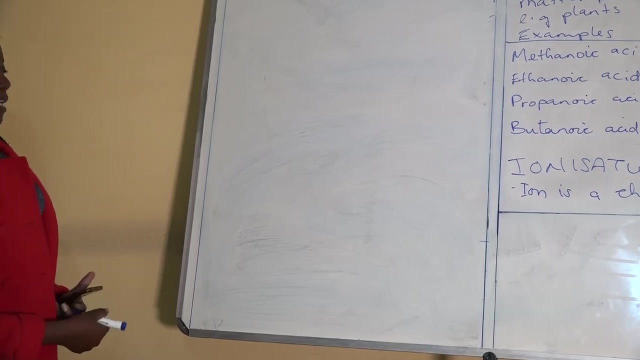 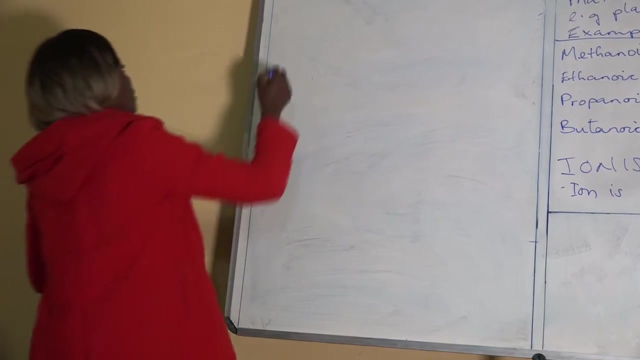 Particular Acid. That Is What We Call Ionization. Alright, That Is What You Can Remember. Okay, So We Pick That From There. Ionization Is The Formation Of Ions, And An Ion Is A Charged Atom. Okay, So To Ionize An Acid Is To Simply Form. 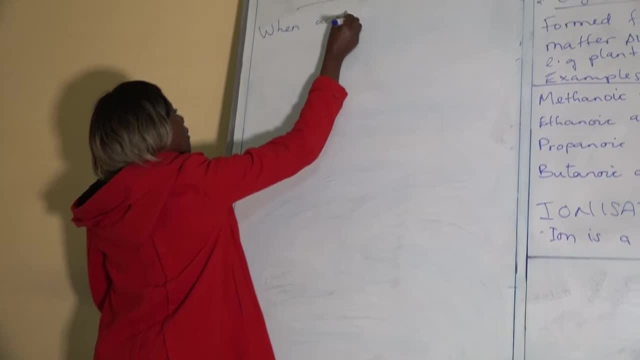 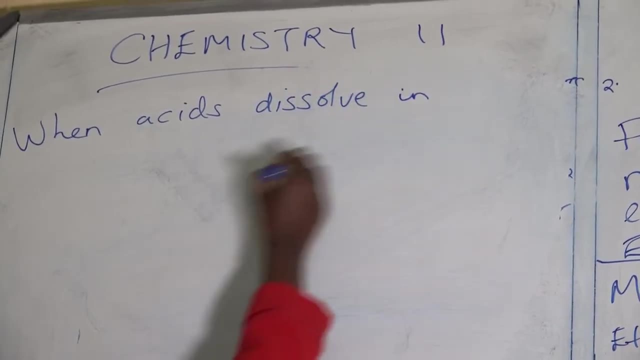 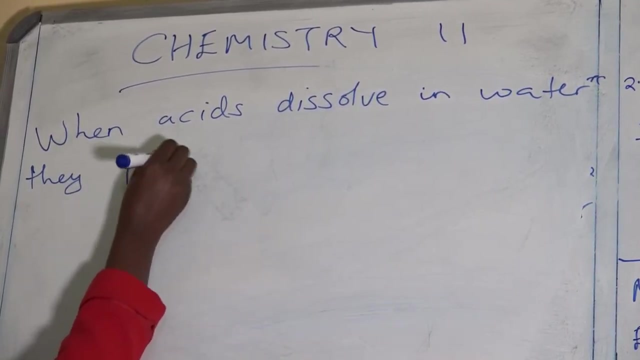 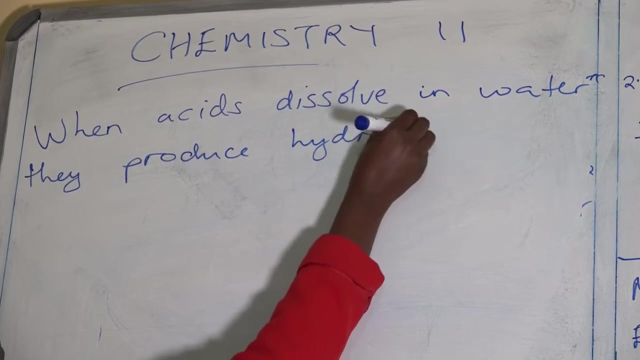 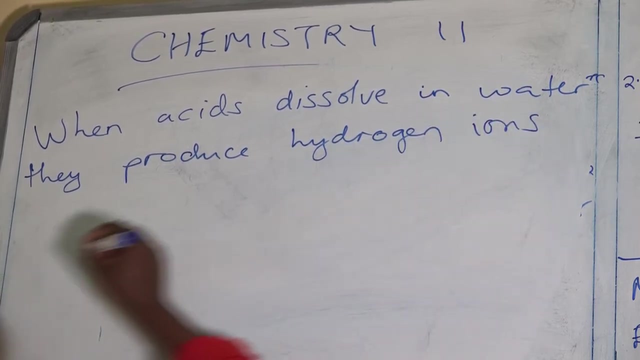 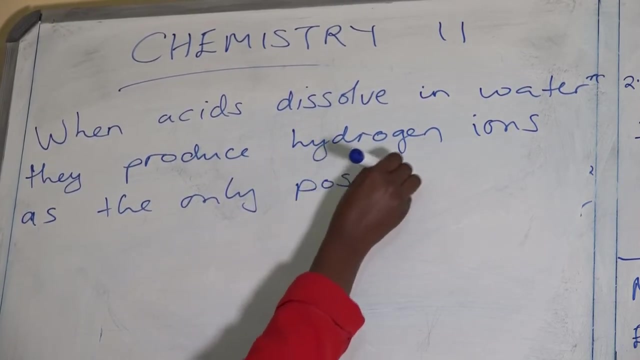 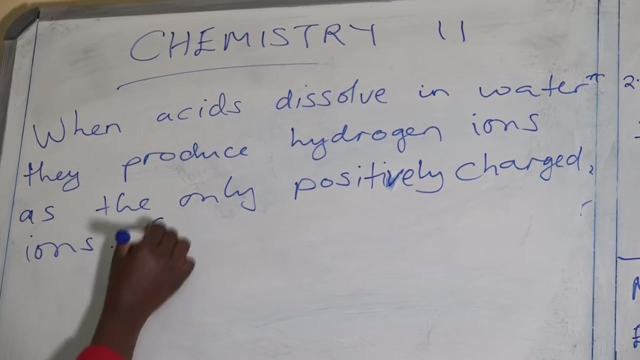 Hydrogen Ions. They Produce Hydrogen Ions. Okay, So Hydrogen As The Only Positively Charged Ions. Okay, This Hydrogen Will Be The Only Positively Charged Ions. Okay, This Hydrogen Will Be The Only Positively Charged. 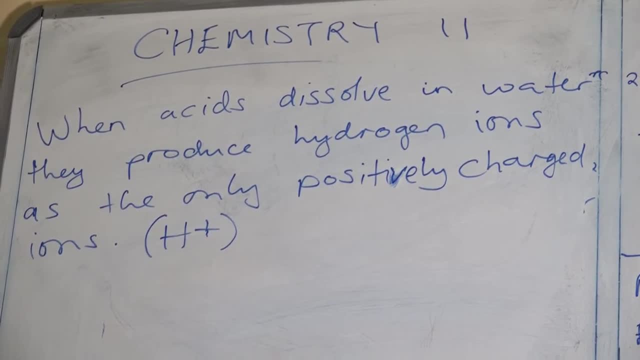 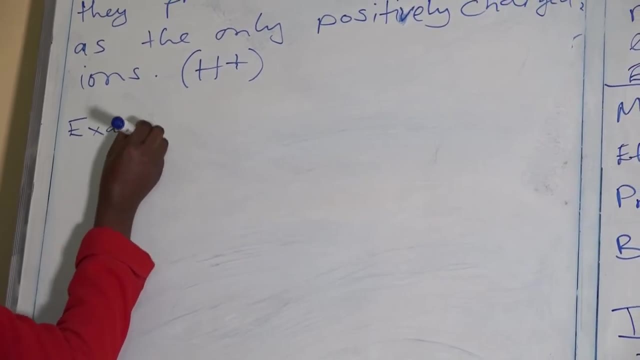 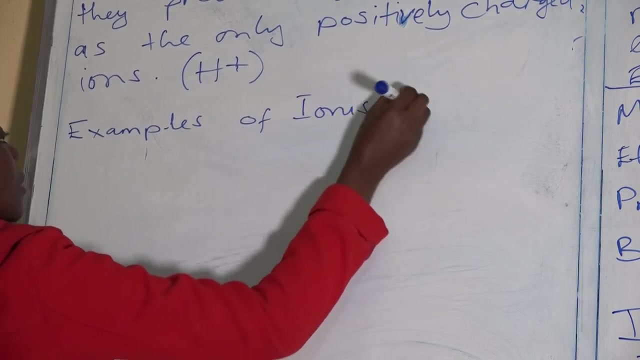 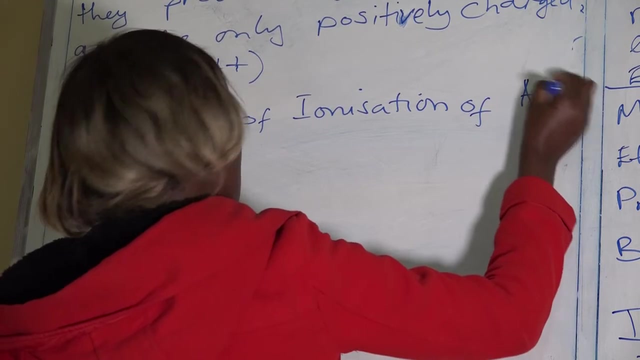 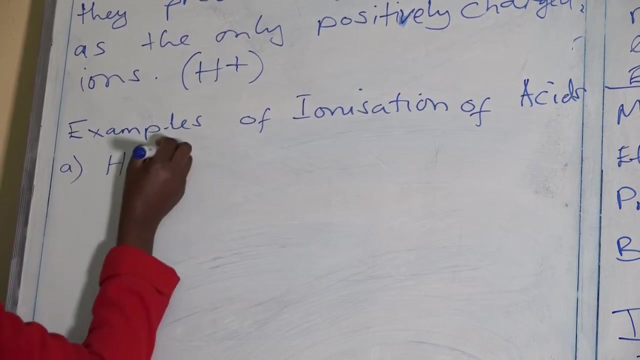 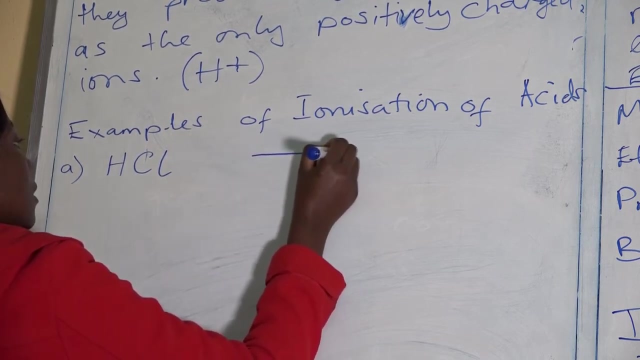 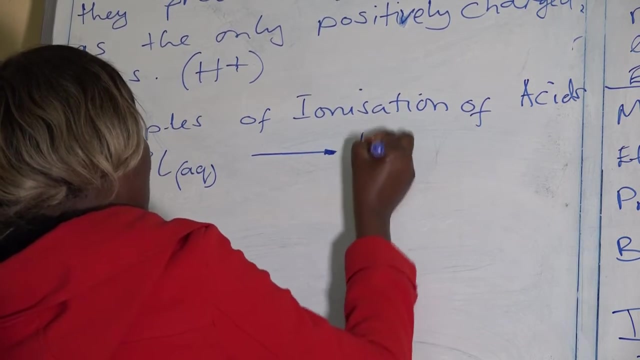 Ions. Let Us Look At Examples Of Ionization. How Are Acids Ionized? Examples Of Ionization Of Acid: We Start With A HCl. Okay, When We Add Hydrogen In Water, It Will Produce Hydrogen Ions As The Only Positively Charged. 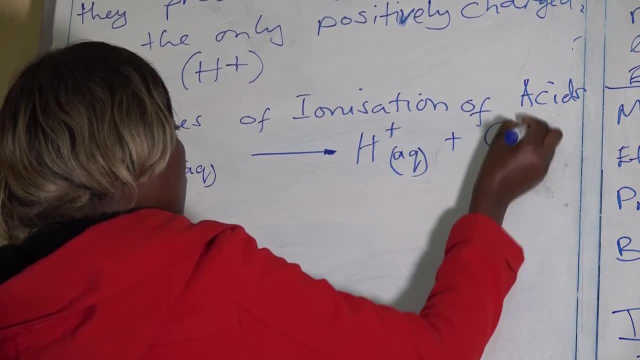 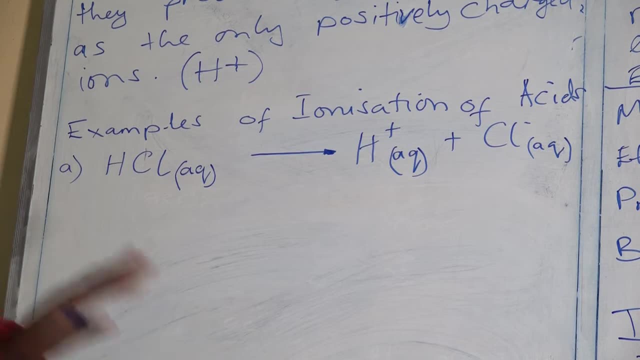 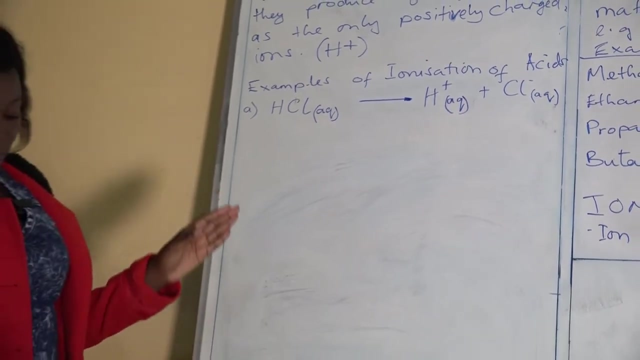 Ions And Chloride Ions, Which We Obviously Do Not Care. The Charge Of Chlorine Acids Is The Production Of The Hydrogen Ion As The Only Positively Charged Ion. We Are Looking At The Production Of The Hydrogen Ion As The Only. 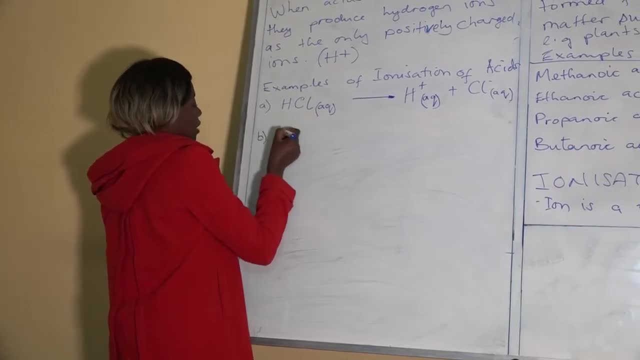 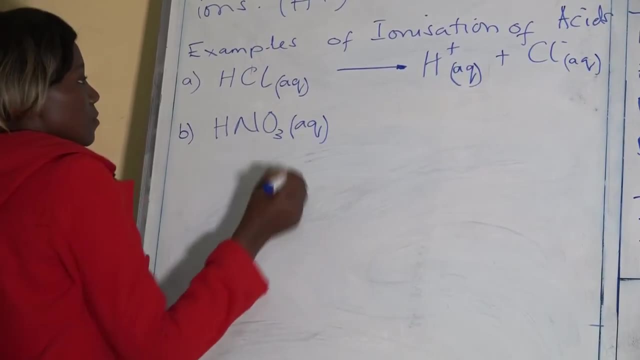 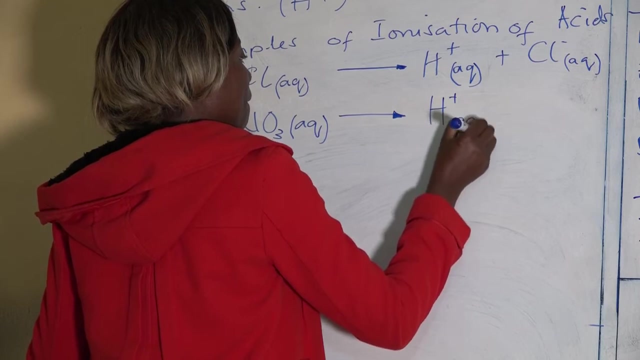 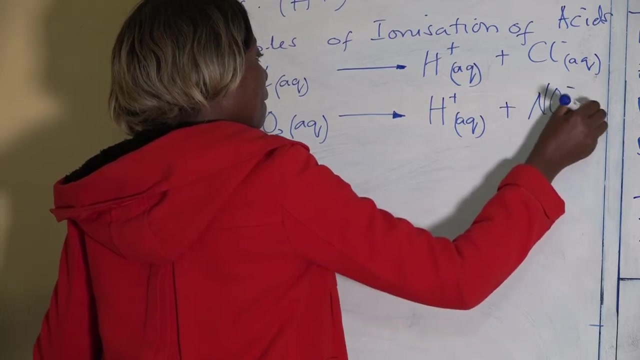 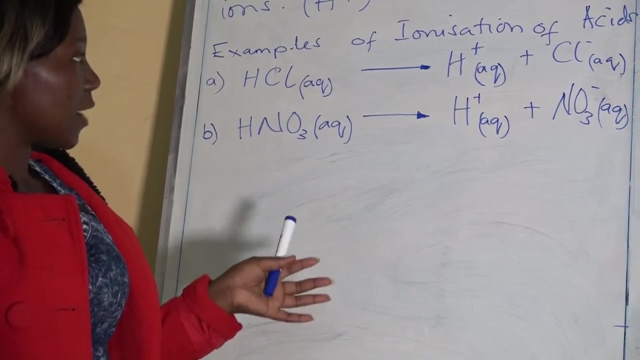 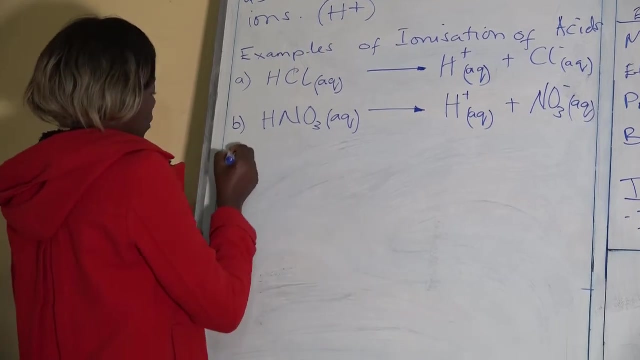 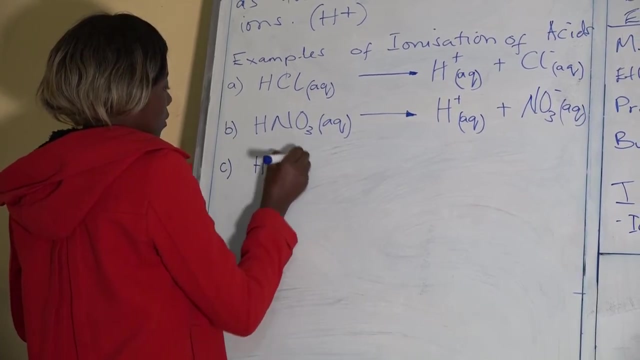 Positively Charged Ion B, Nitric Acid, Will Also Follow Suit. Hydrogen Ions Are Going To Be The Only Positively Charged Ions. What About Phosphoric Acid? Hydrogen Ions Are Going To Be The Only Positively Charged Ions. What About Phosphoric Acid? 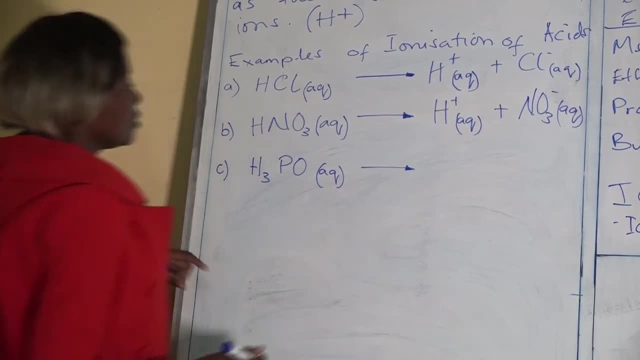 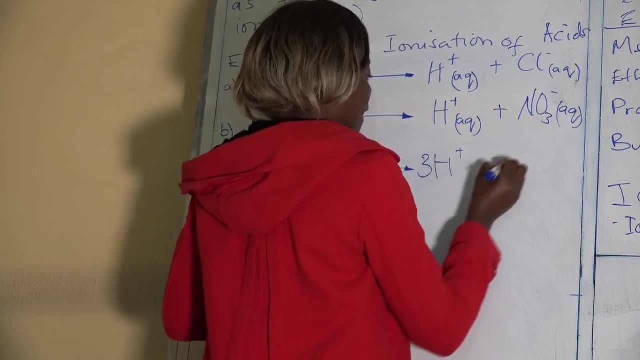 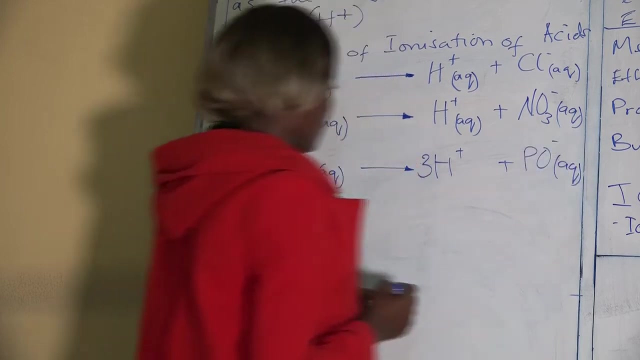 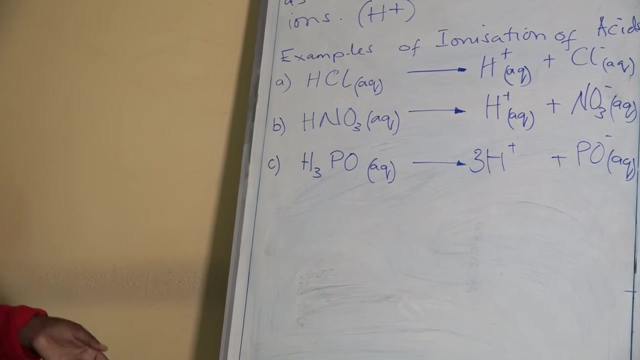 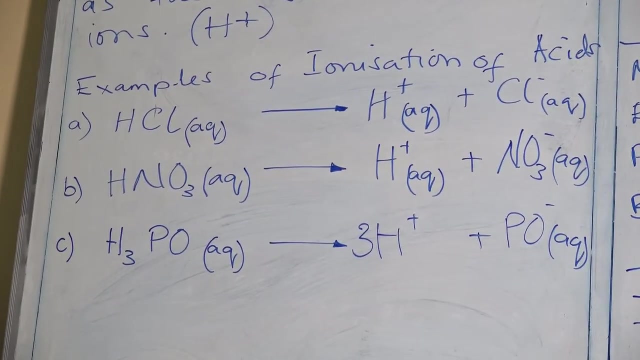 When It Dissolves In Water We Will Have Hydrogen Ions. So From Here You Can See Clearly That After Ionizing These Acids We Can Tell That Clearly: Only Hydrogen Is Positively Charged, only the hydrogen is positively charged. the other parts of the reaction or 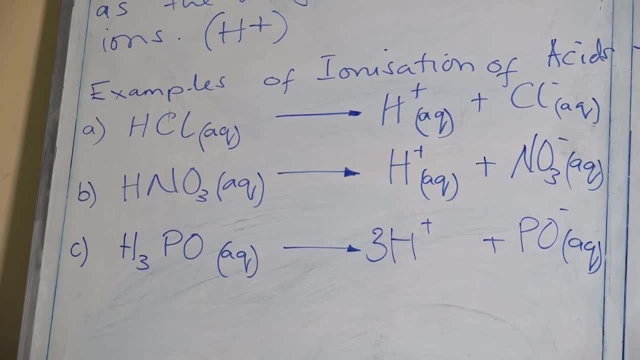 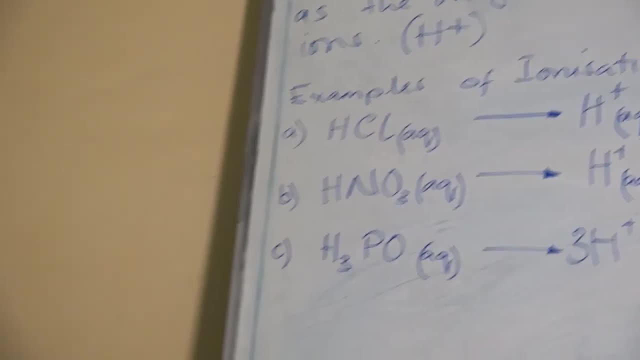 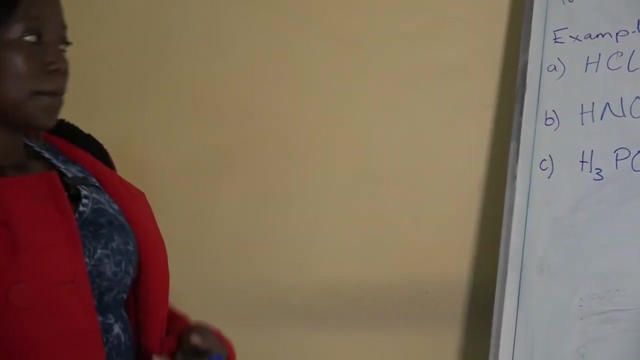 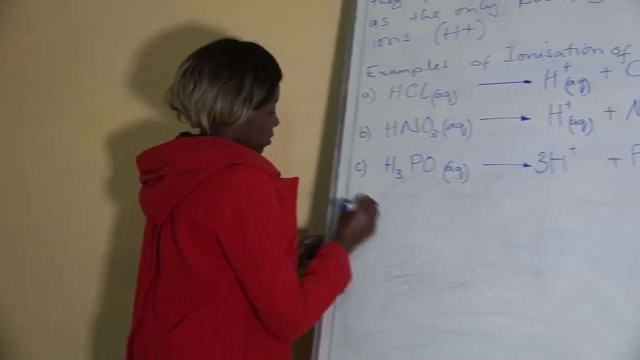 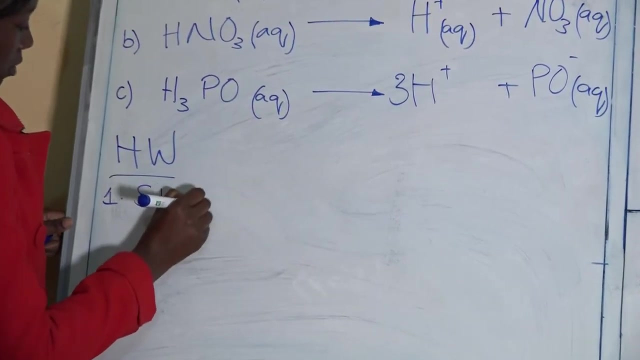 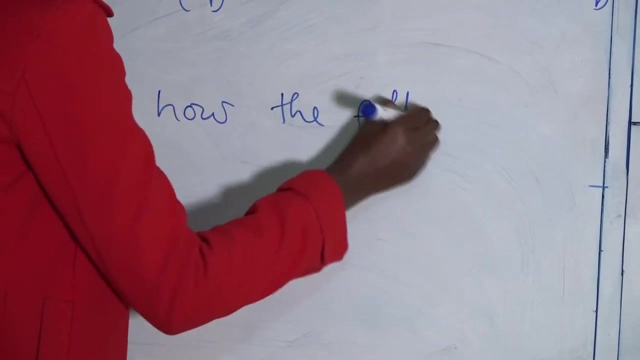 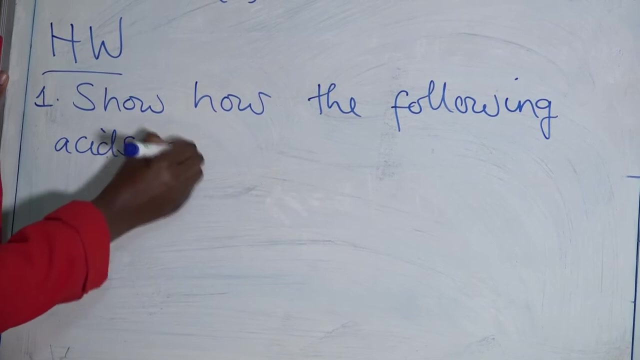 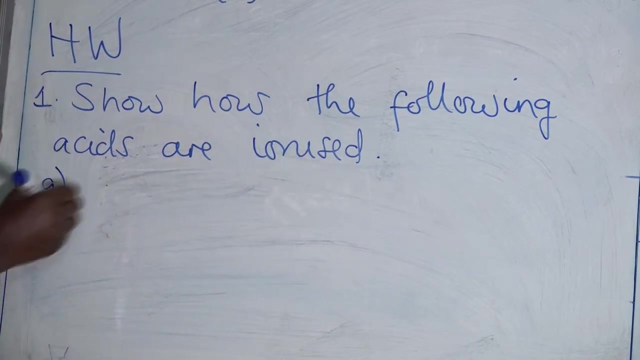 rather, the mineral part of the acid dissolves and comes out negative, negatively charged. only the hydrogen ion is positively charged. okay, so this is how acids are ionized. you can as your homework. okay, you can show how the following acids are ionized: okay, sulfuric acid. 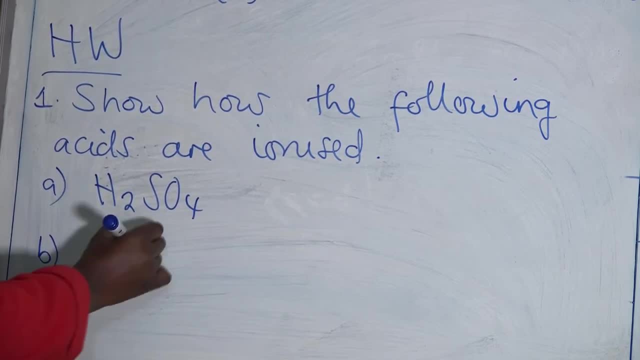 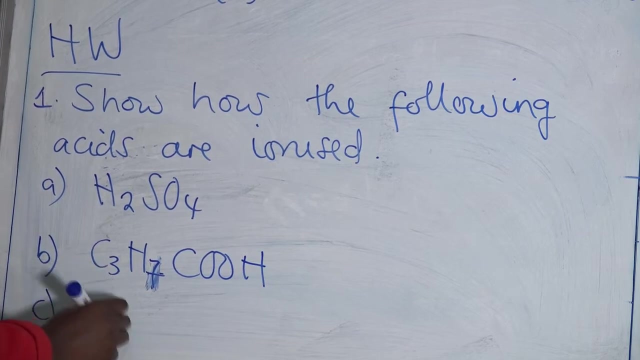 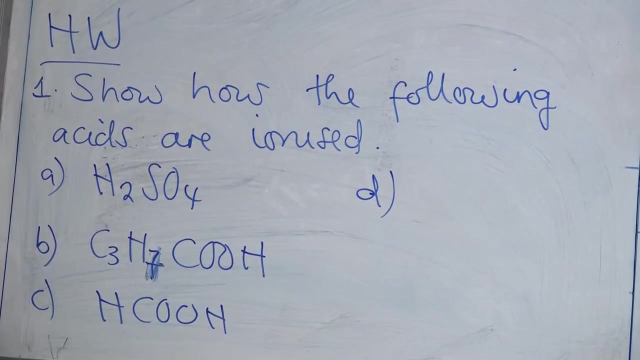 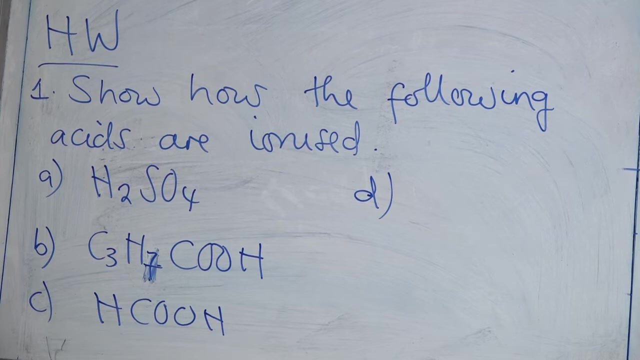 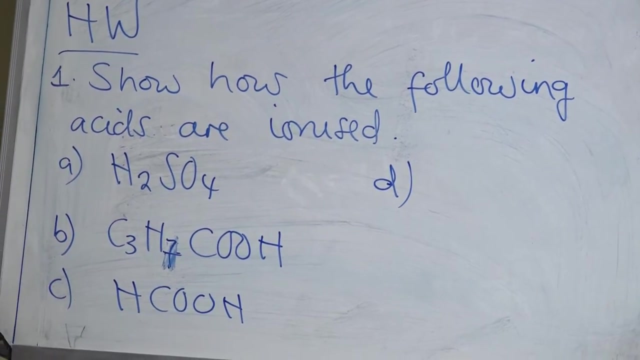 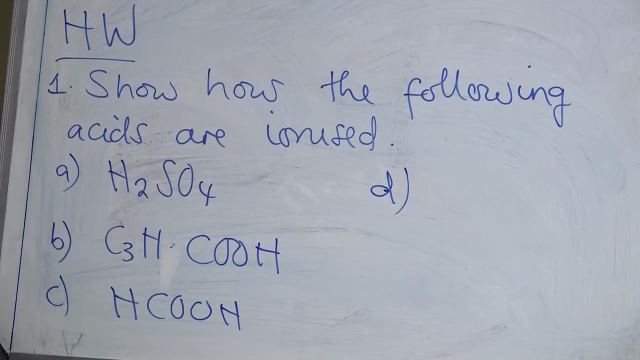 butanoic acid, okay. methanoic acid and tea, let's have okay. okay, these three enough. show how sulfuric acid and methanoic acid are ionized. butanoic acid and methanoic acid are ionized. show how sulfuric acid, butanoic 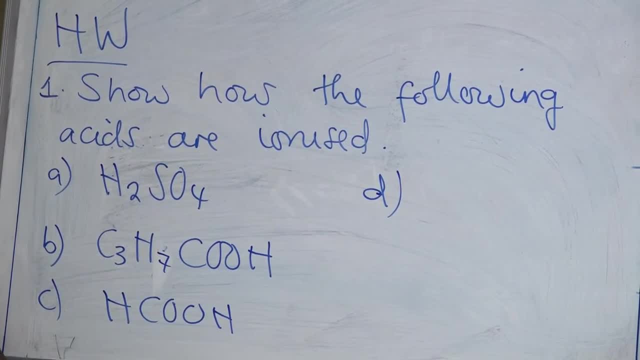 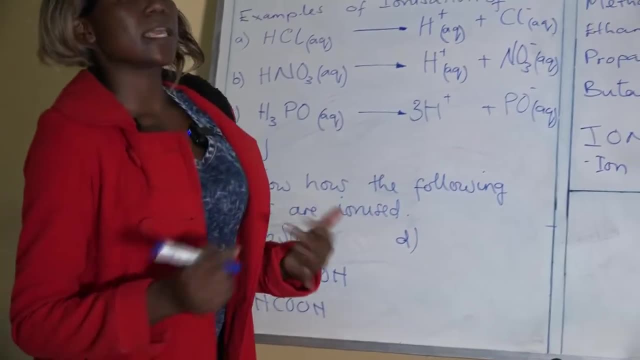 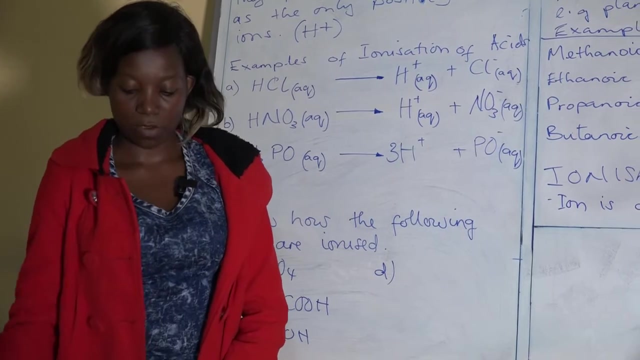 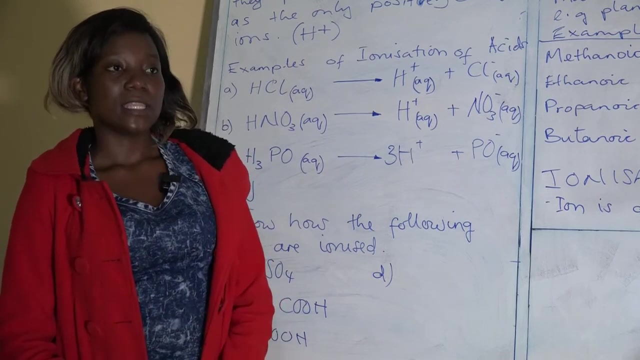 acid and methanoic acid are ionized. okay, having looked at what an acid is, i mentioned that an acid is a chemical substance which, when dissolved in water, produces hydrogen ions as the only positively charged ions. there are two types of acids. the first one is a mineral acid. this one is formed from metals. this one is formed. from metals, and hence the term mineral acid. so it is formed from the combination of the metal and hydrogen ions and which, when ionized, will produce a negatively charged particle and a hydrogen ion being the only positively charged ion. the other type of acid we looked at is an organic acid. this is 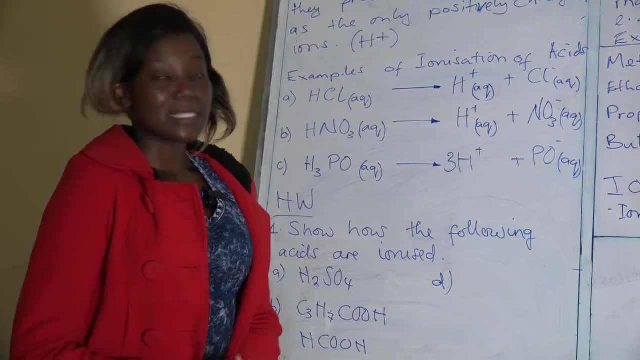 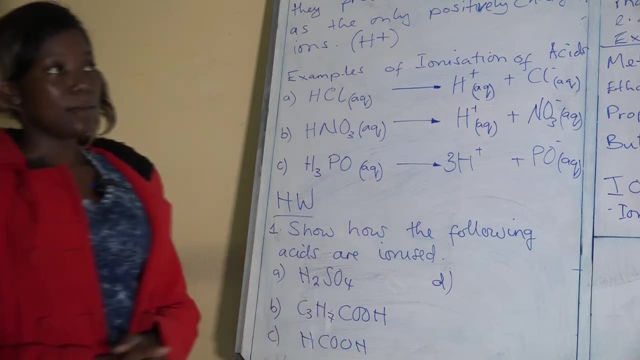 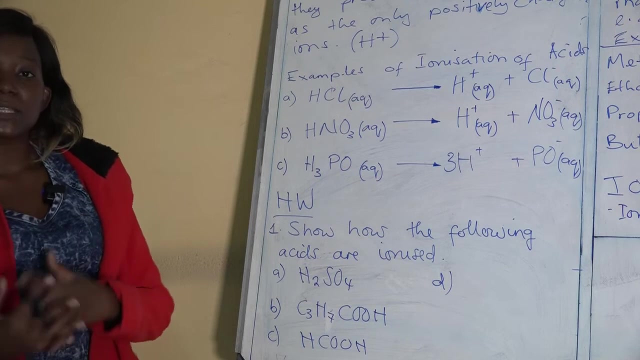 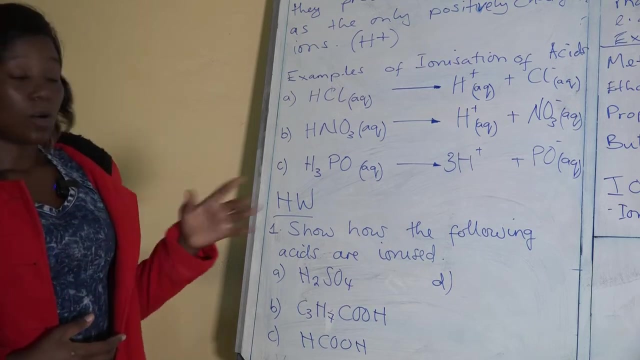 formed from natural organic matter, such as that of living things, for example, plants. okay, so the acid we find in lemons, the acid we find in oranges, is an organic acid. examples are methanoic acid, carbonic acid, butanoic acid, propanoic acid and ethanoic acid. all these acids on the board, this part of 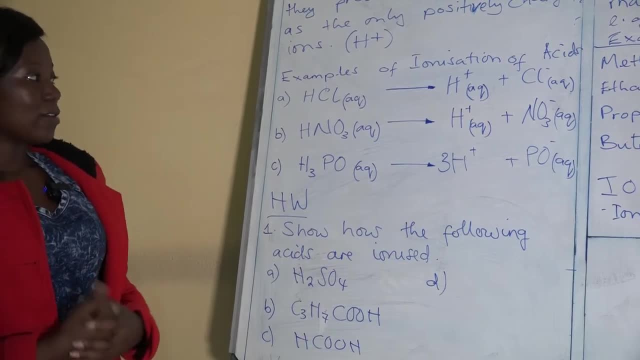 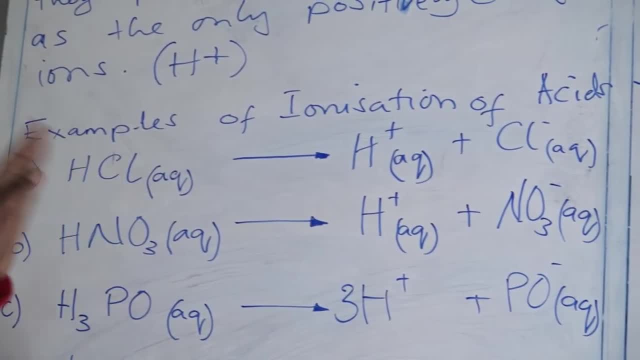 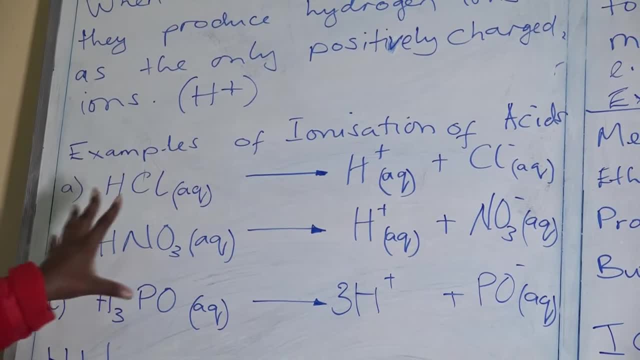 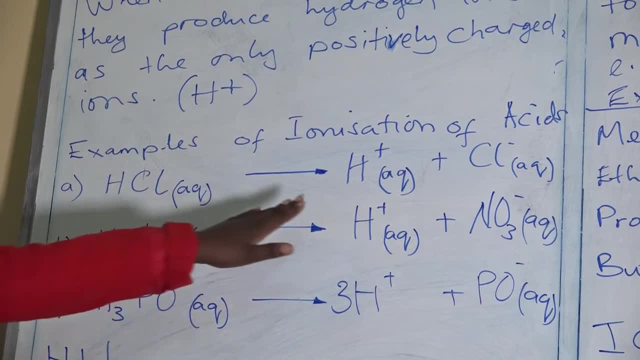 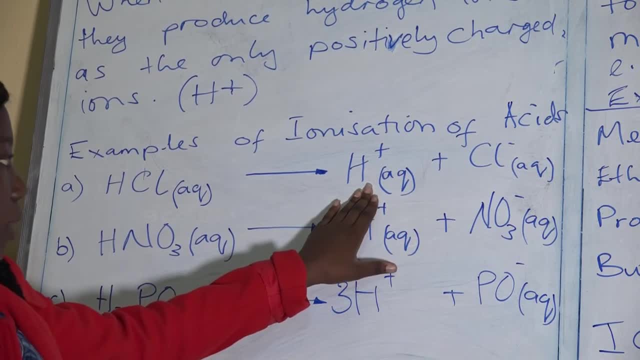 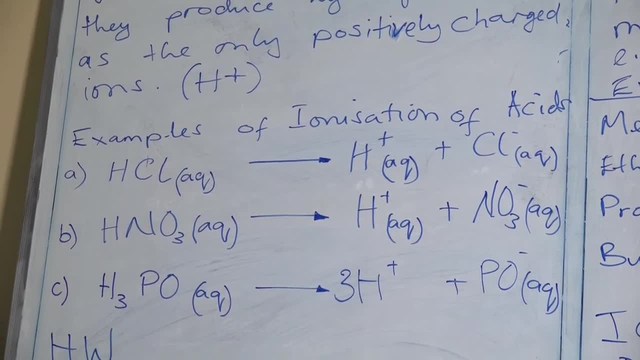 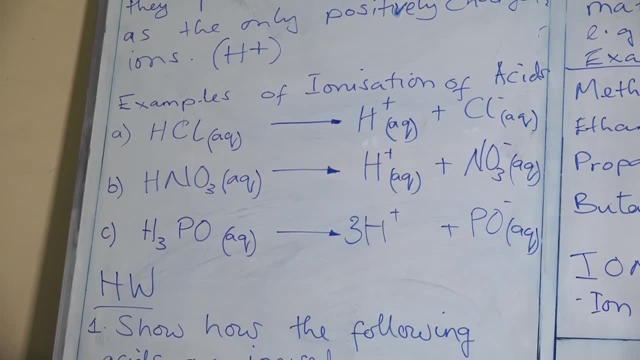 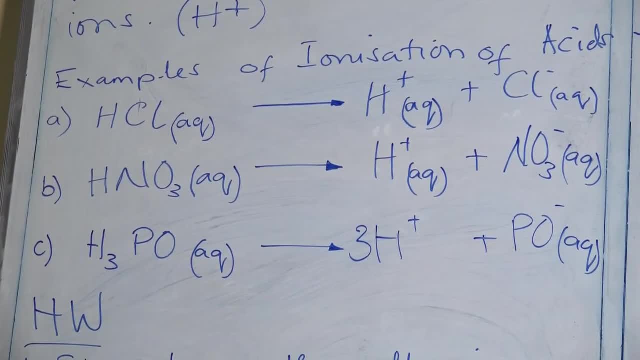 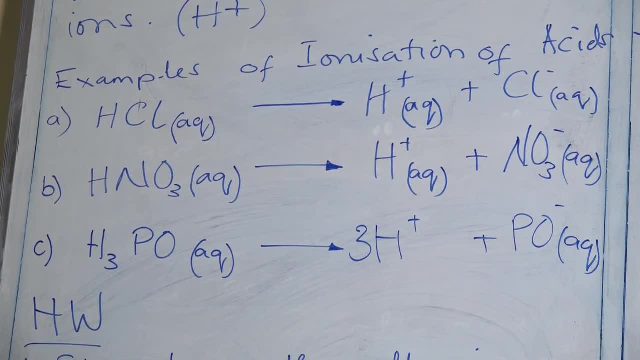 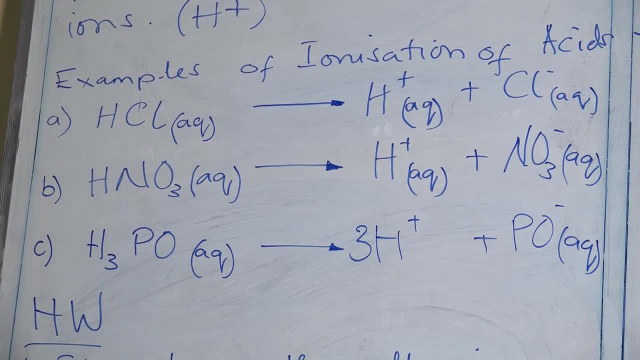 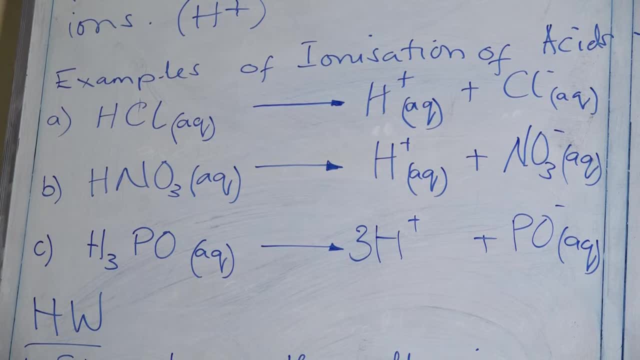 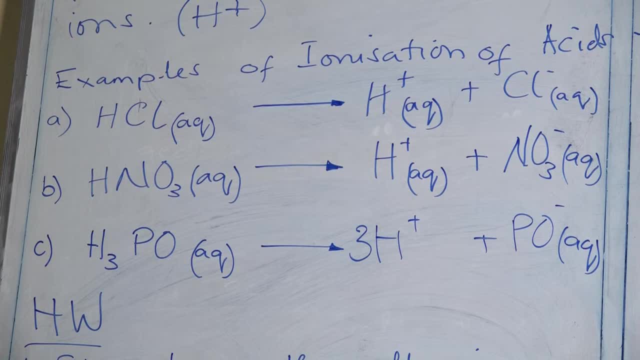 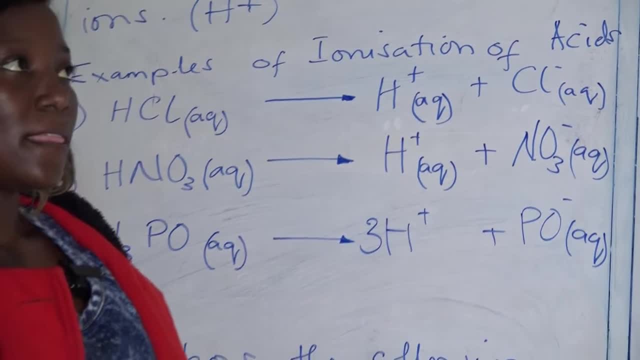 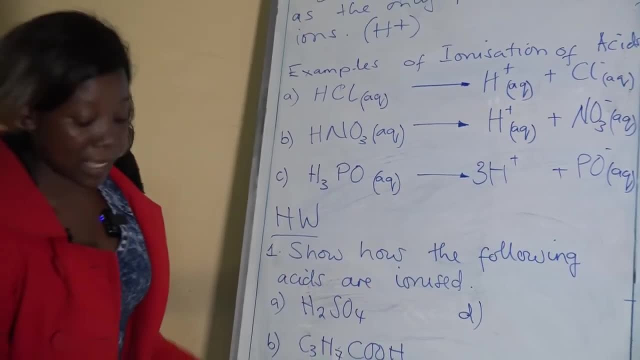 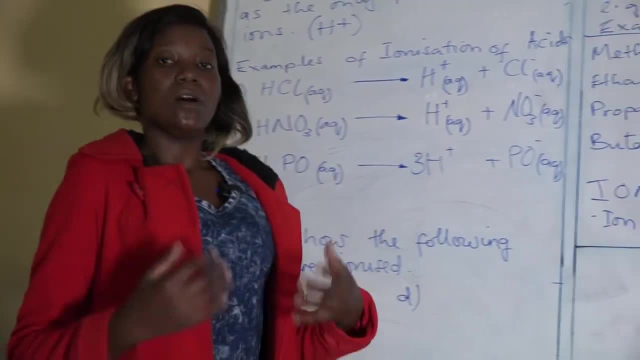 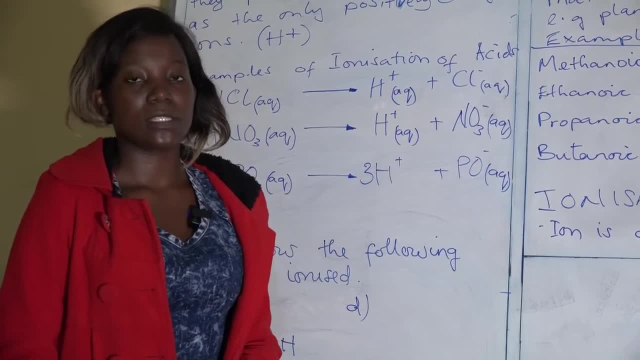 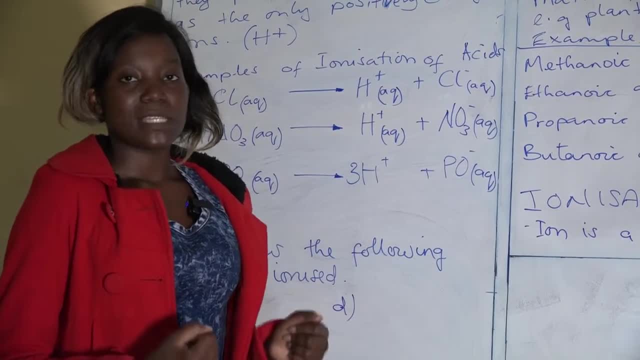 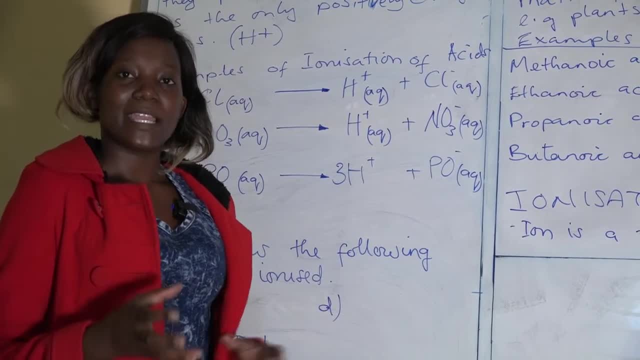 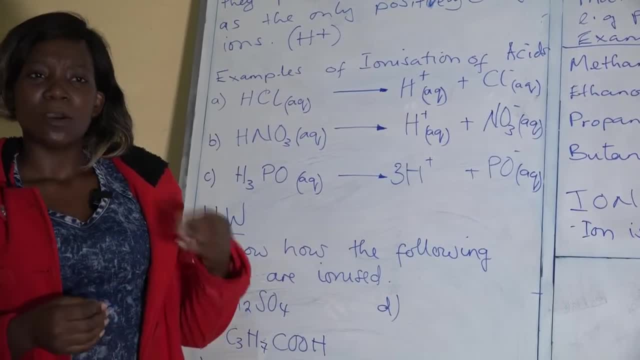 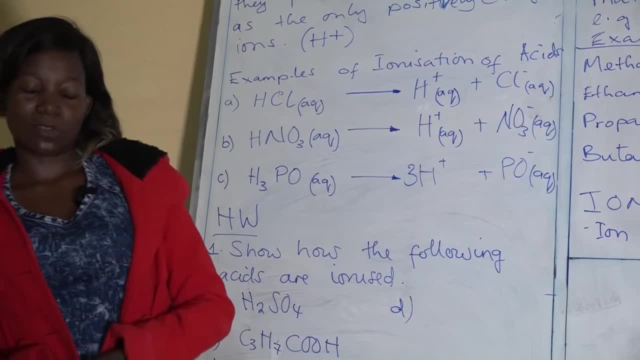 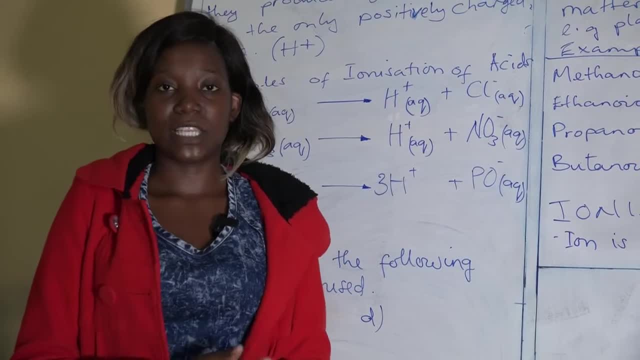 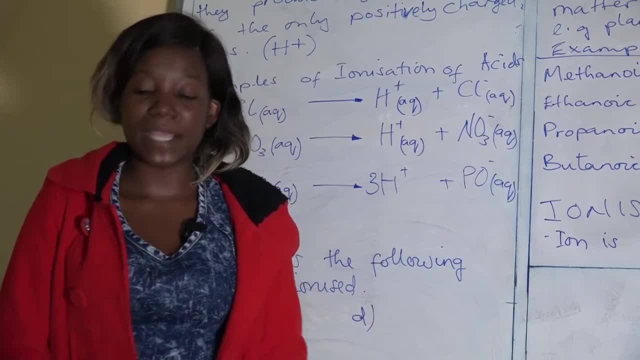 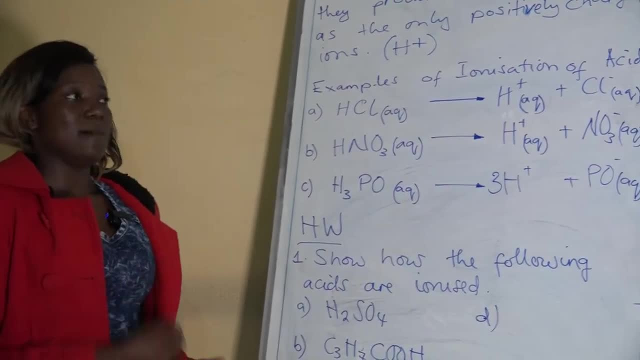 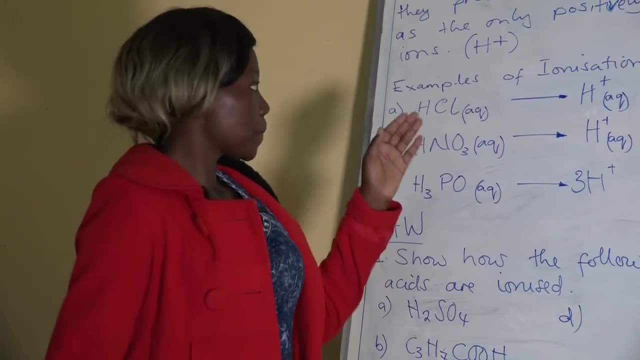 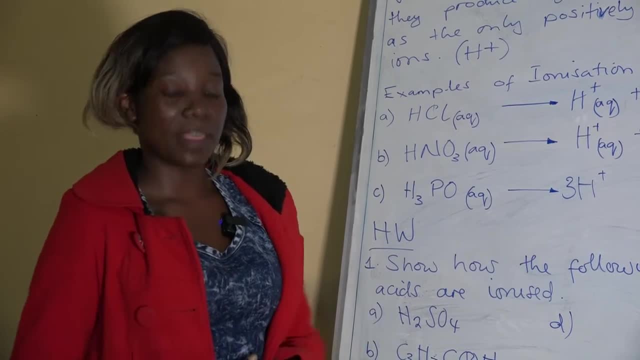 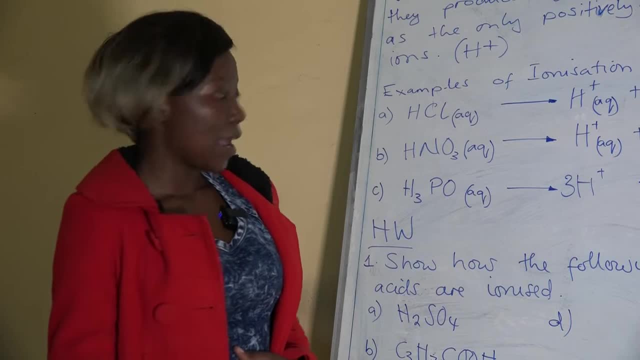 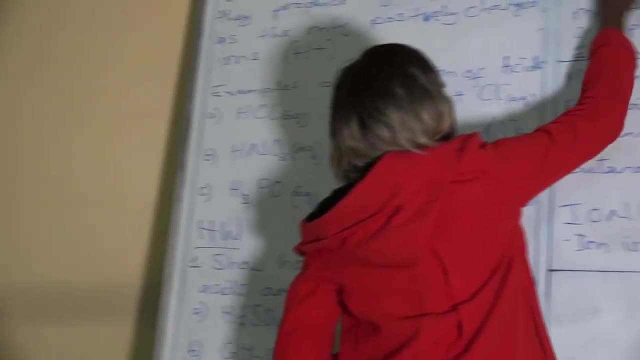 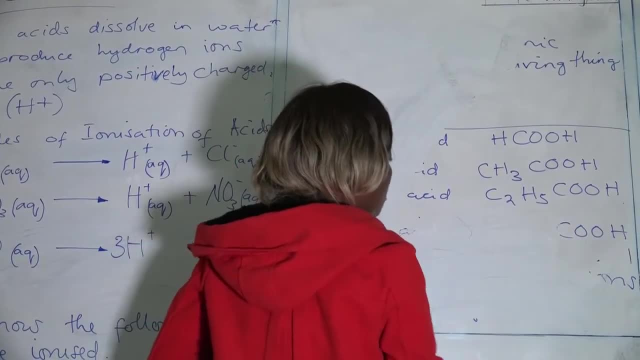 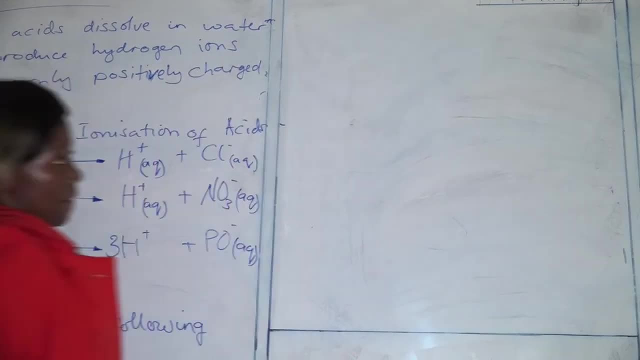 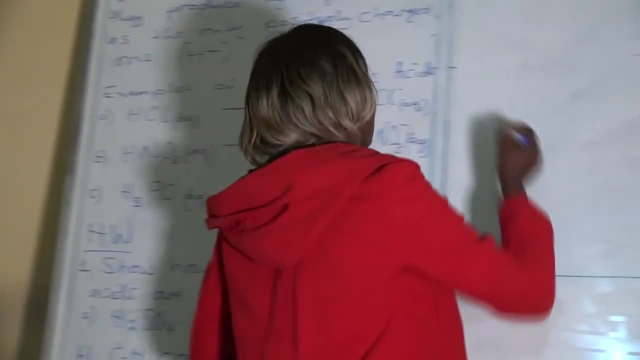 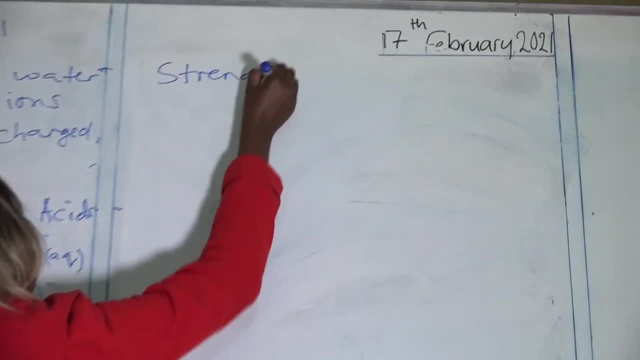 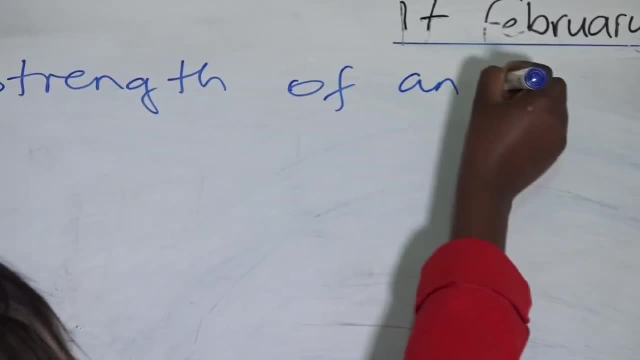 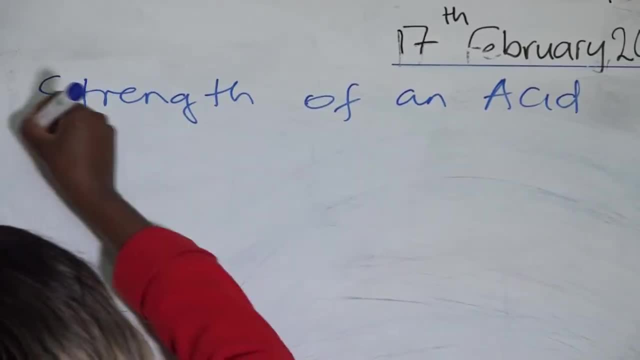 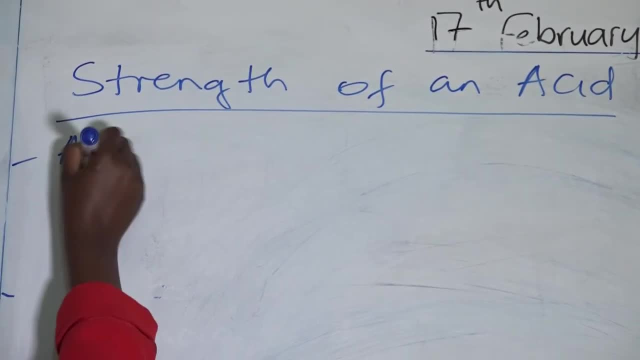 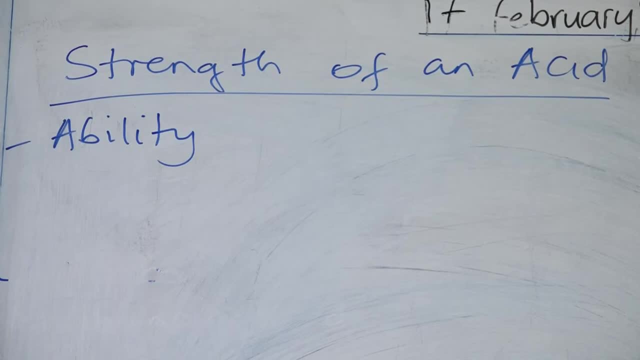 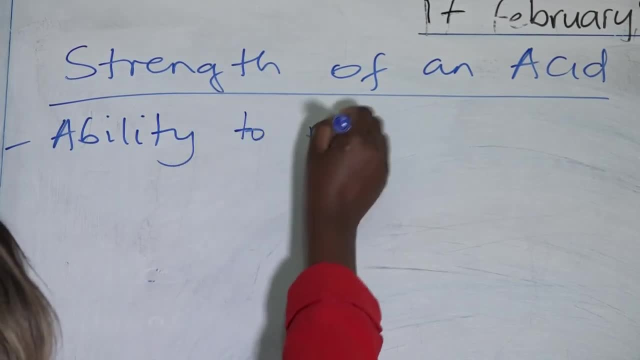 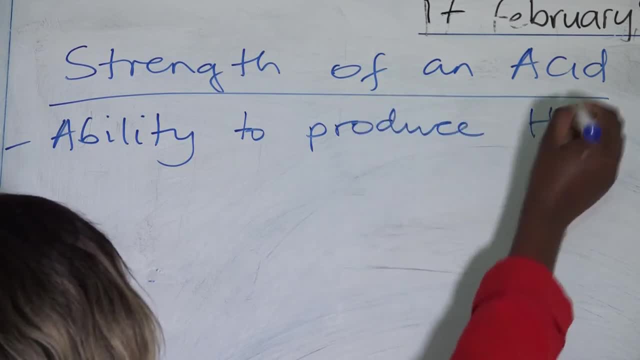 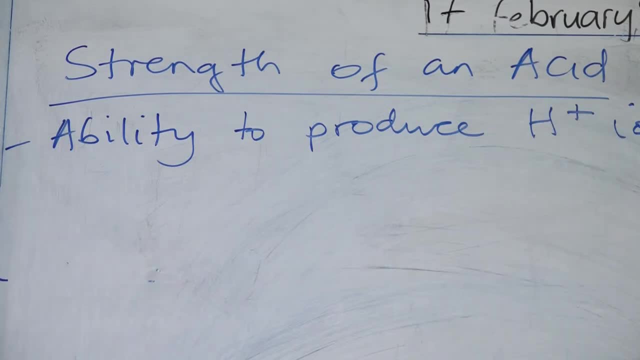 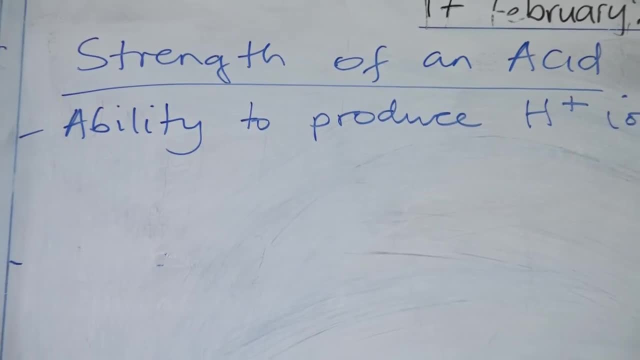 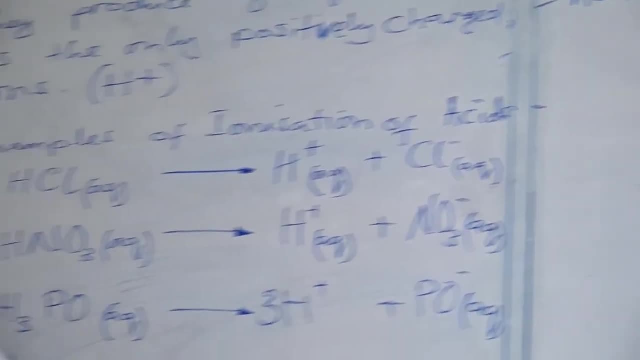 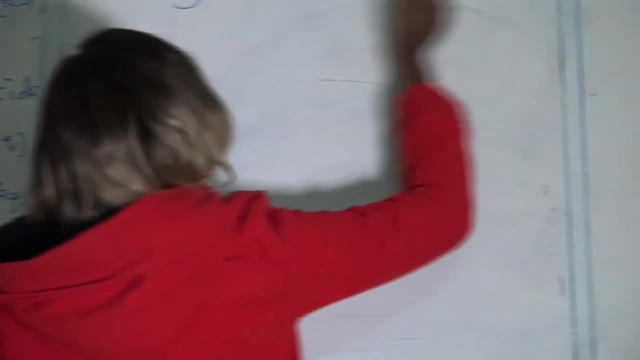 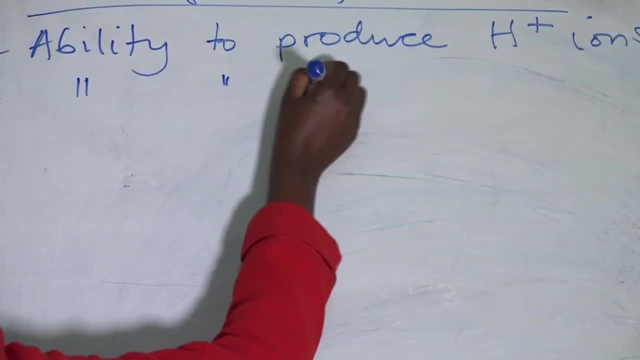 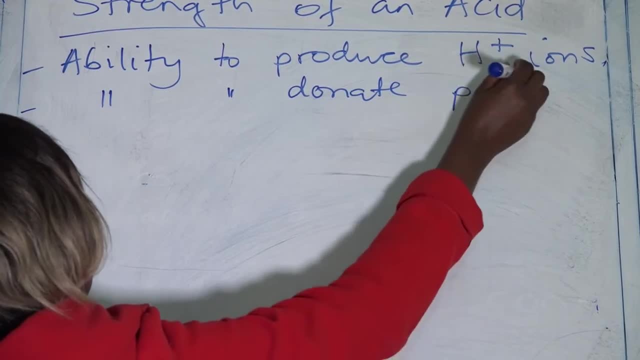 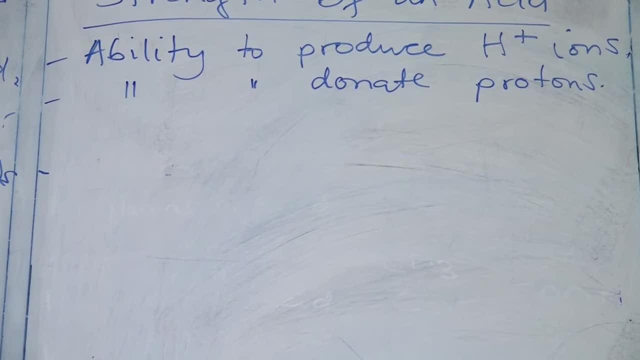 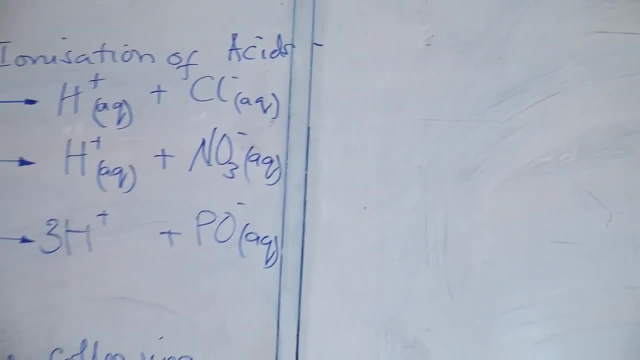 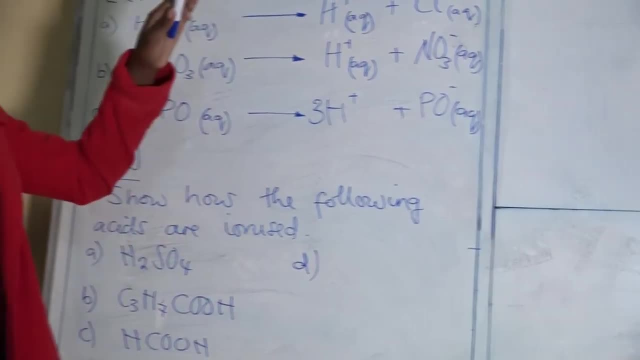 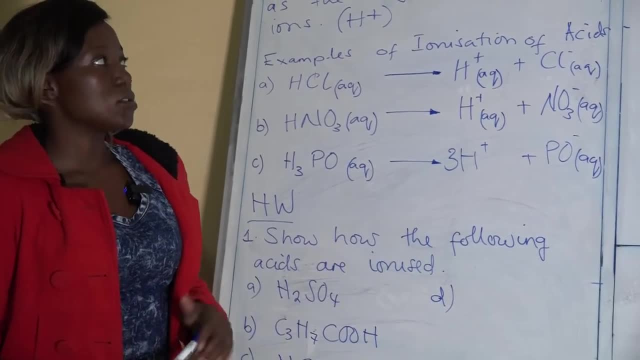 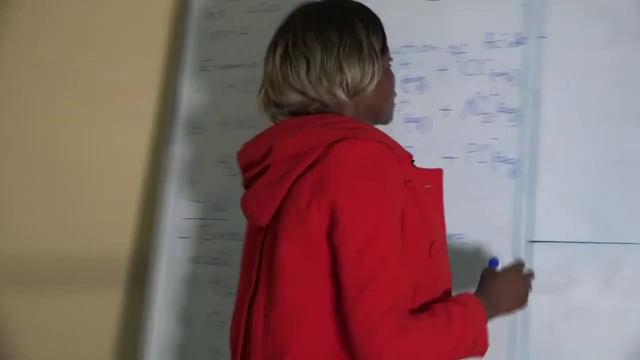 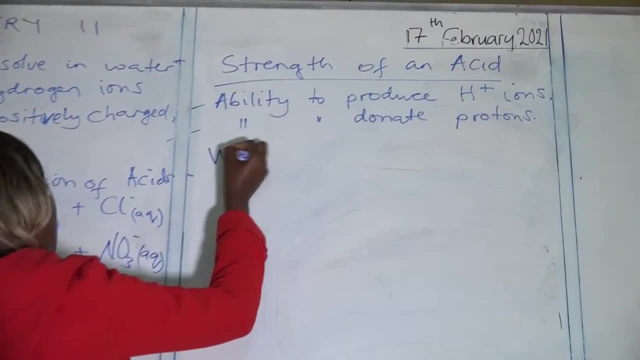 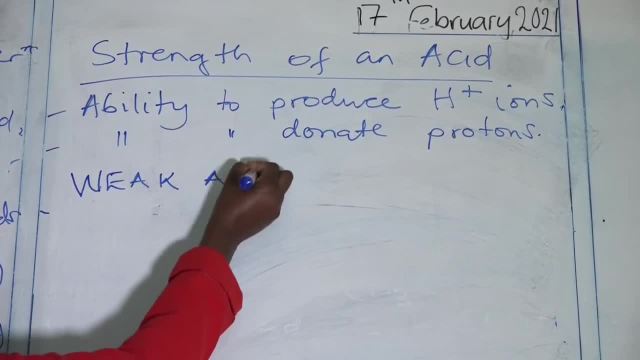 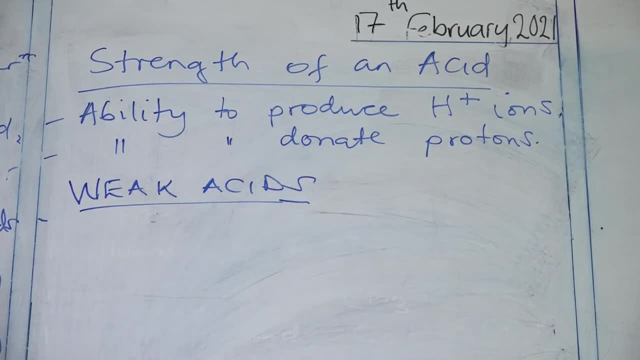 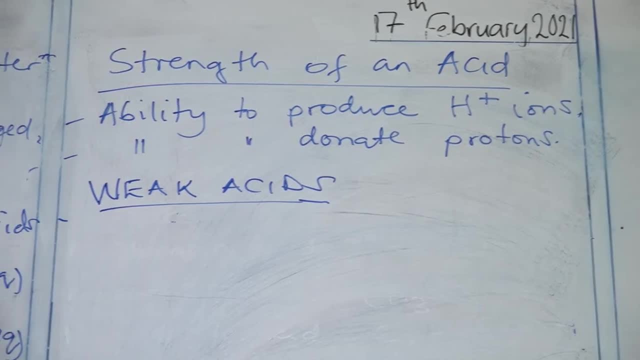 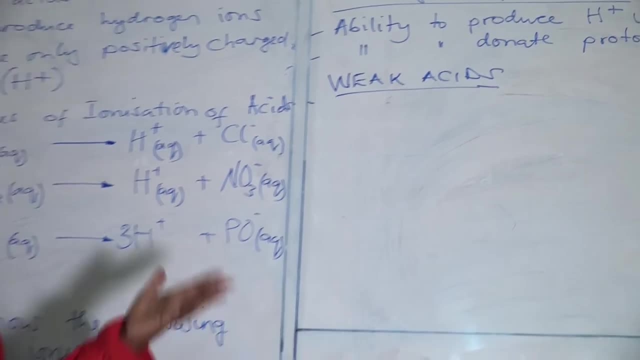 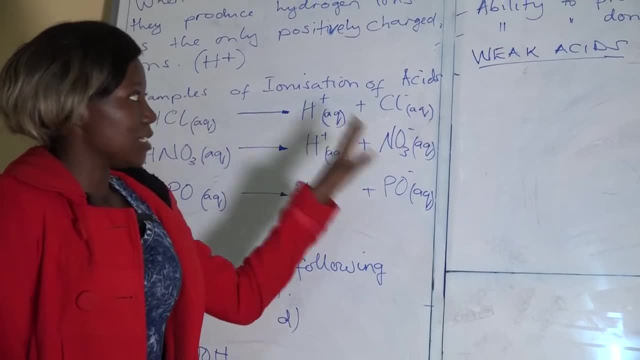 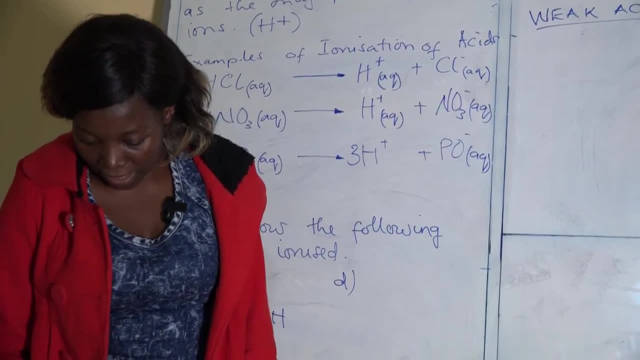 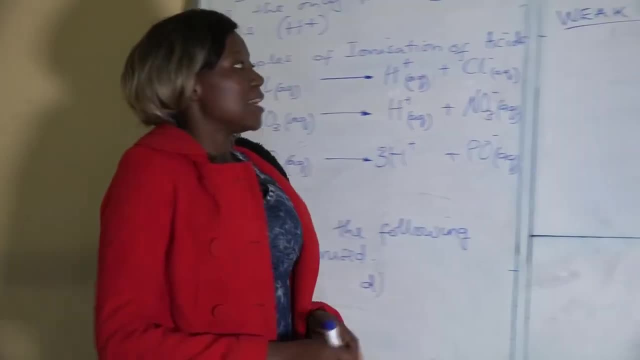 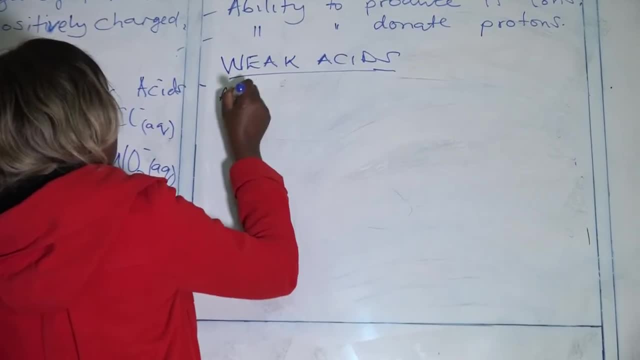 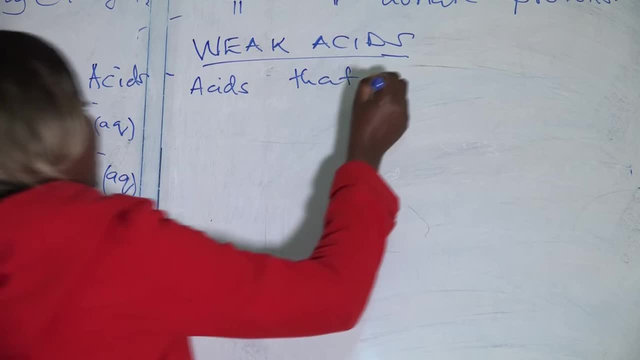 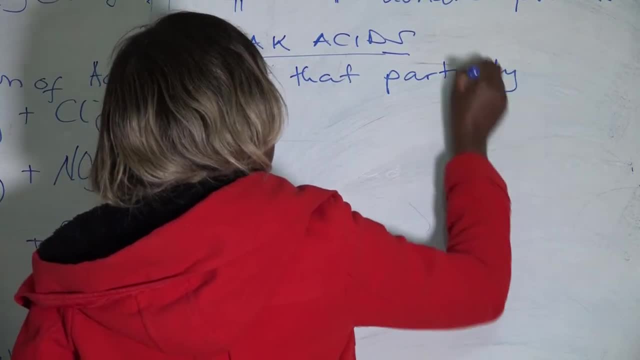 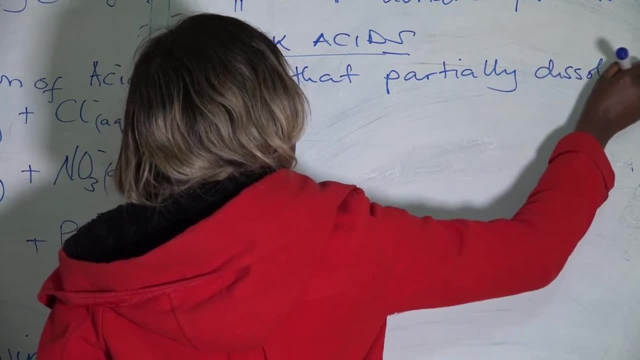 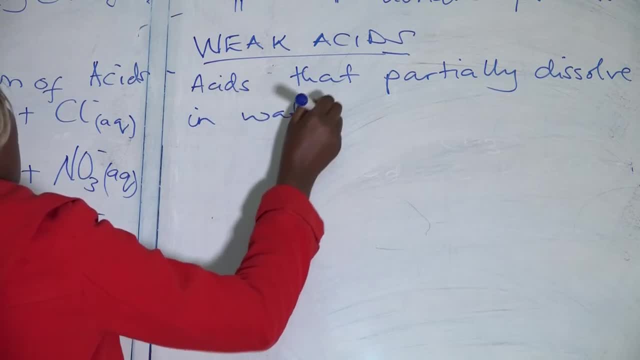 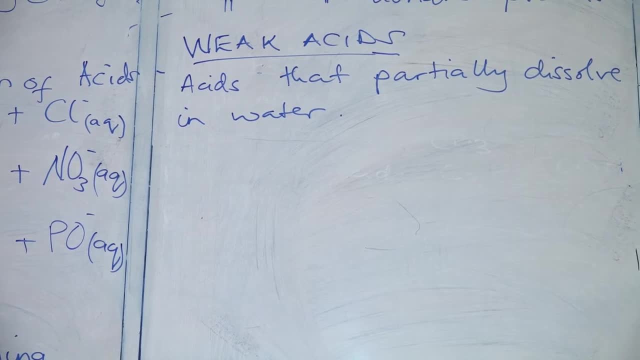 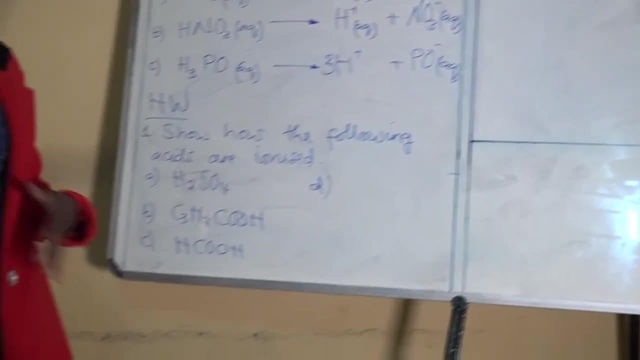 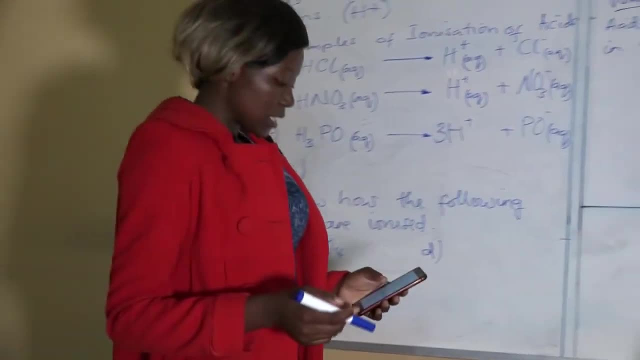 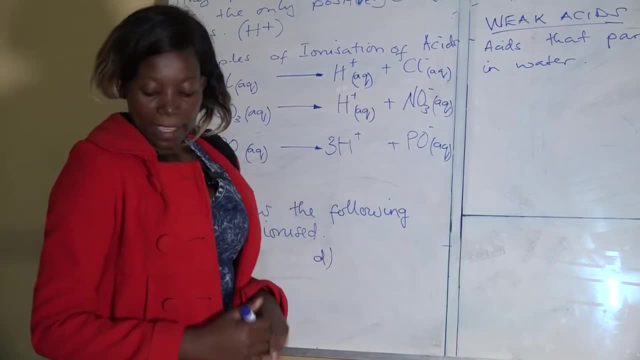 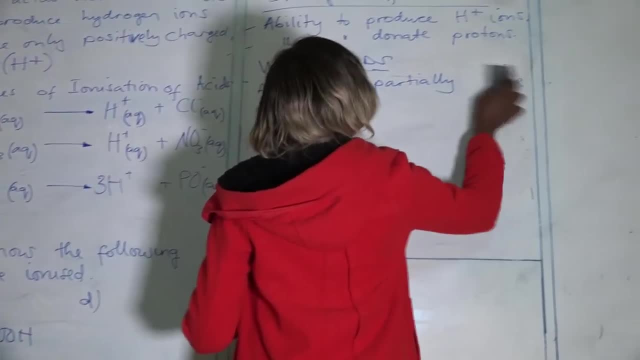 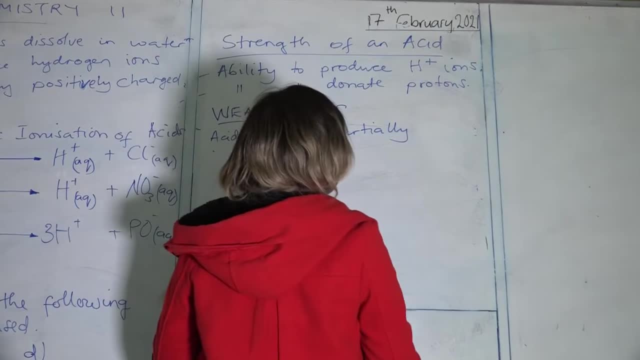 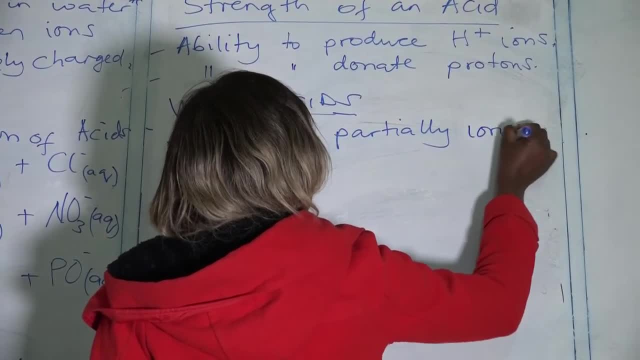 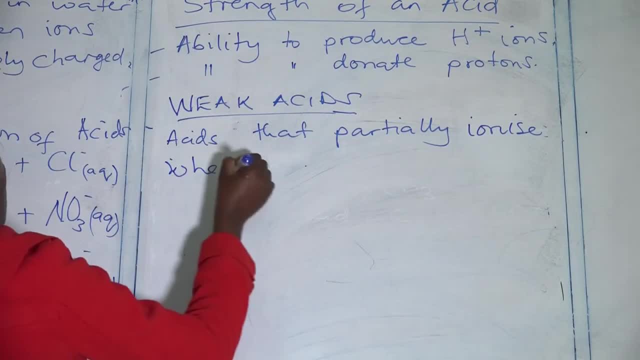 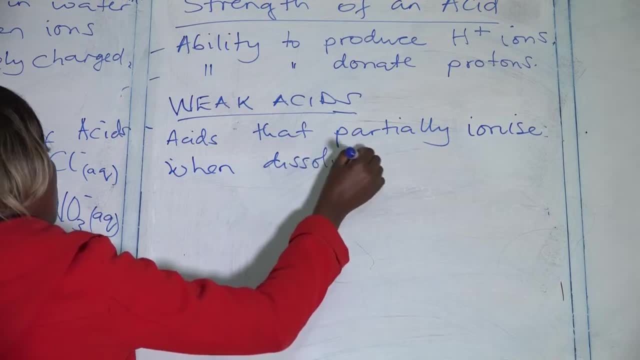 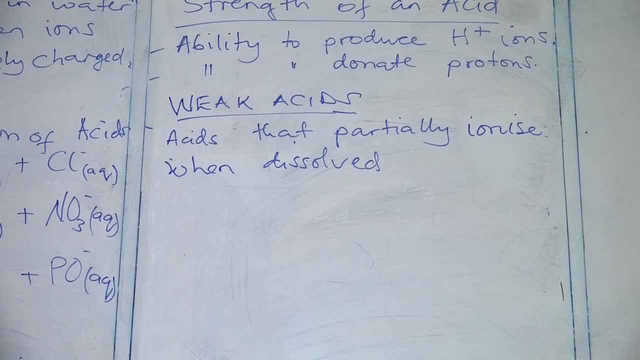 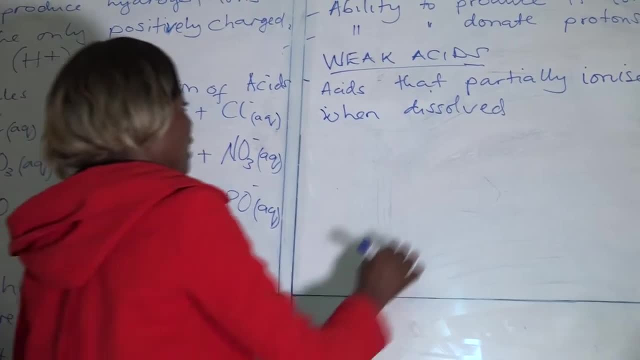 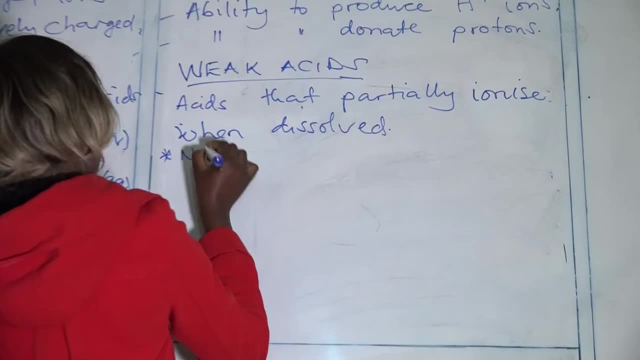 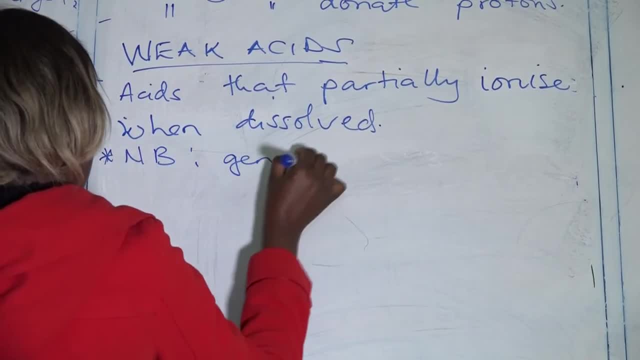 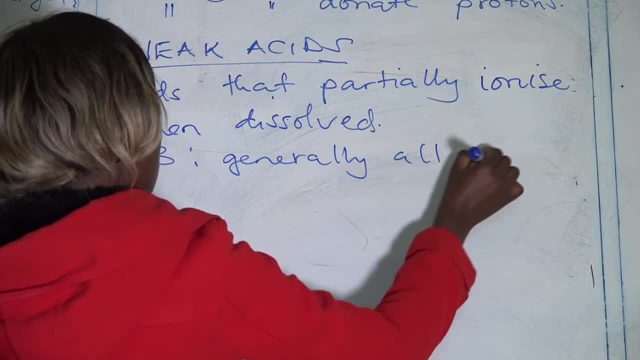 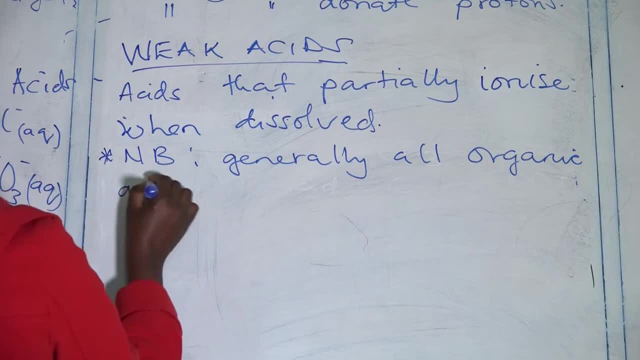 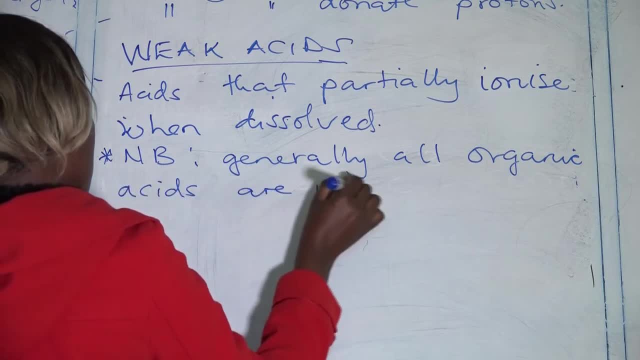 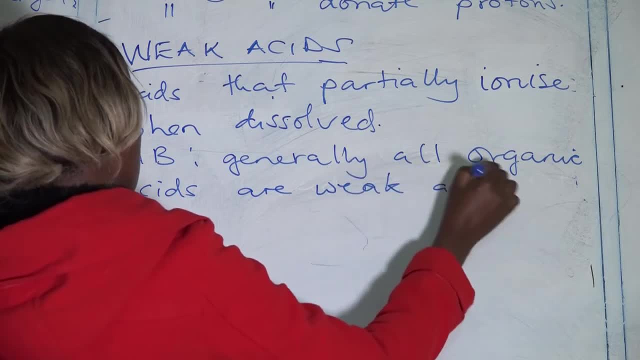 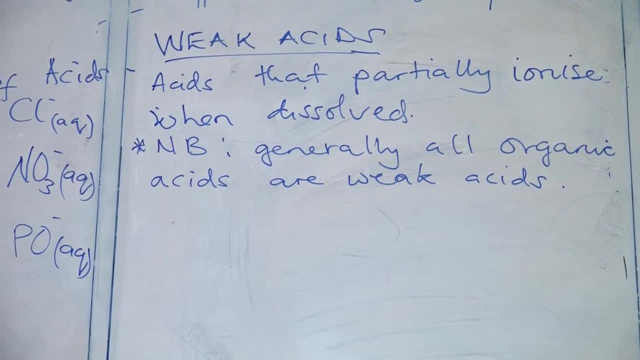 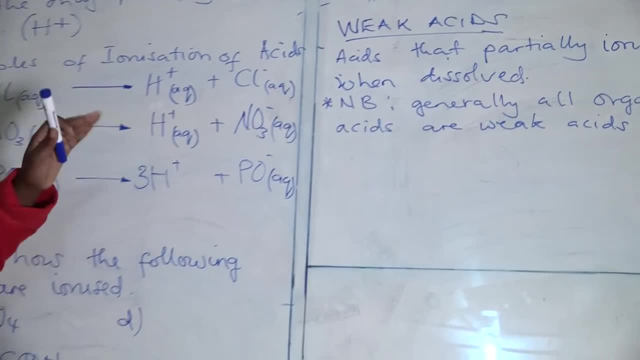 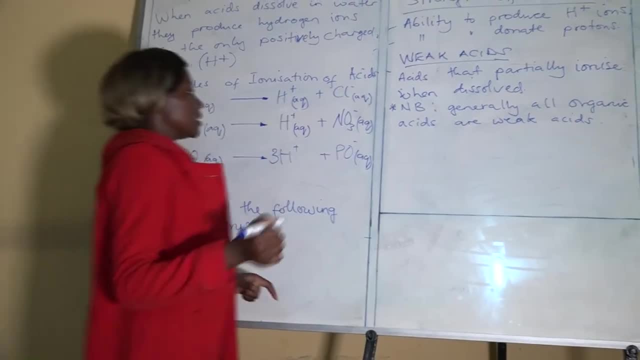 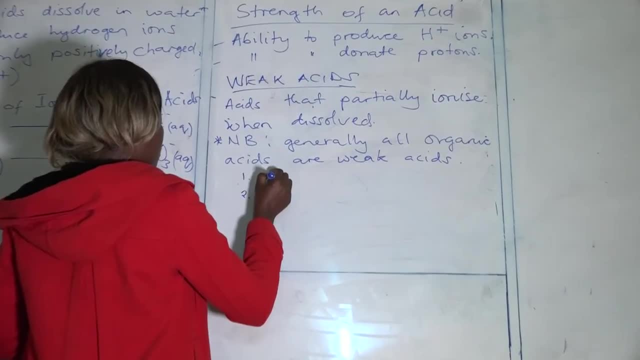 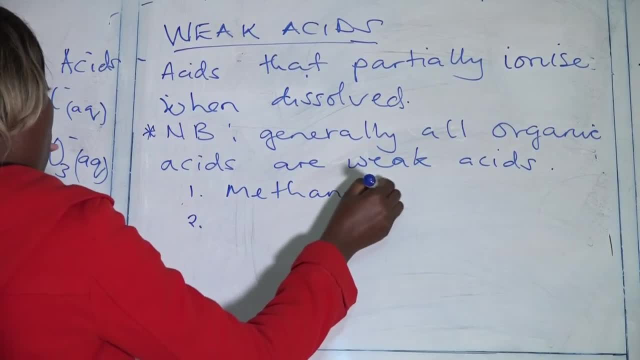 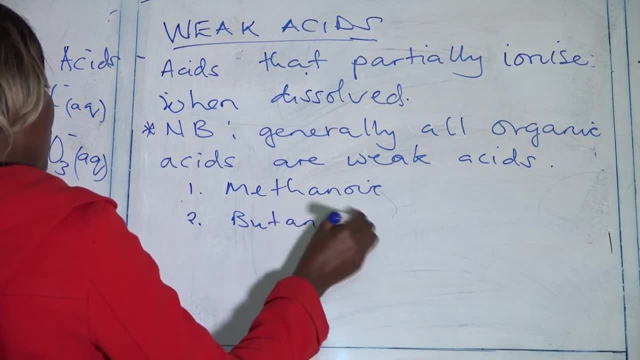 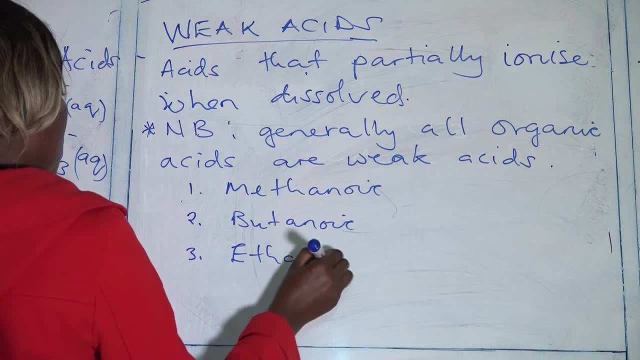 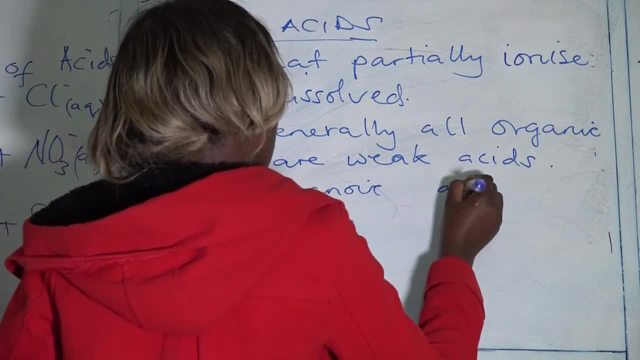 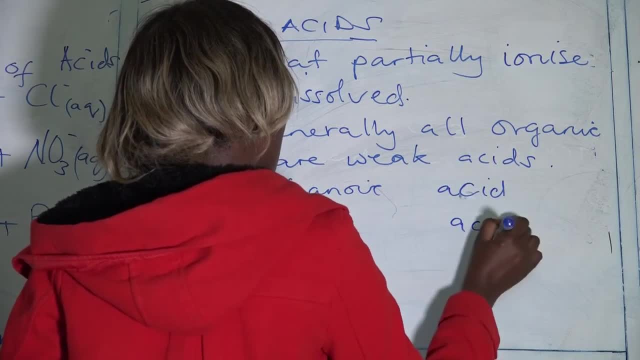 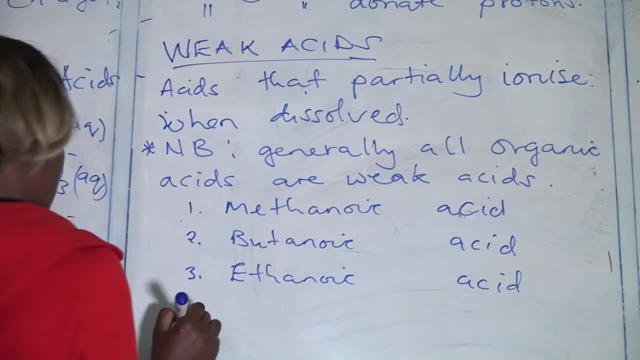 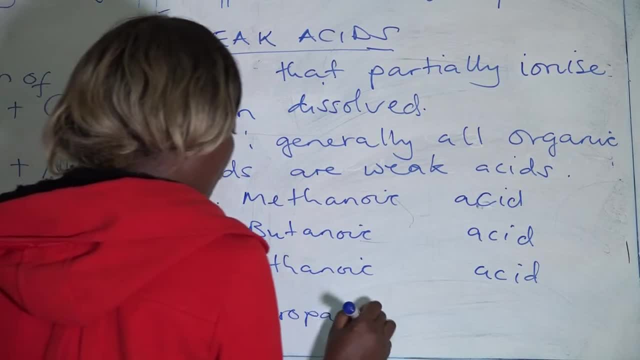 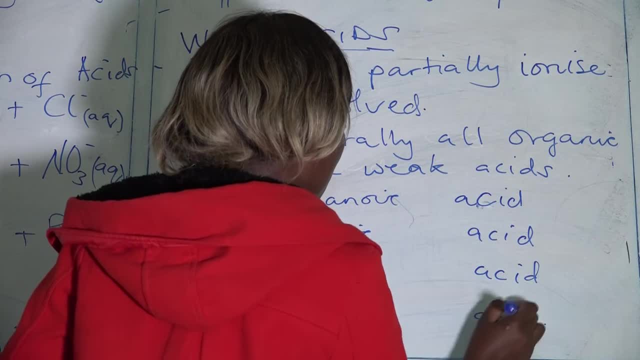 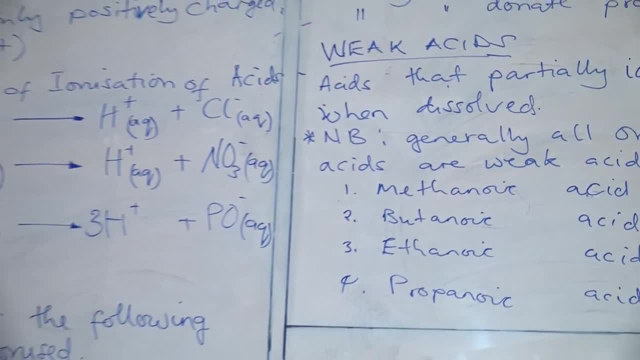 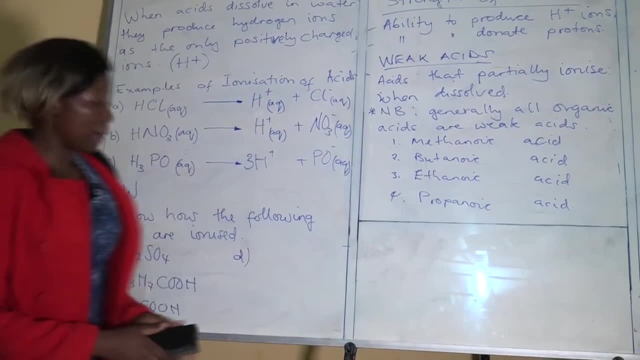 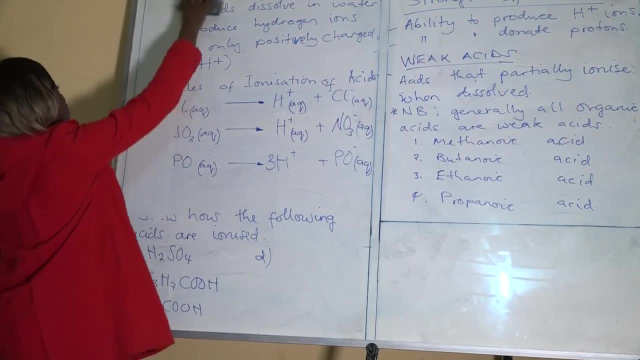 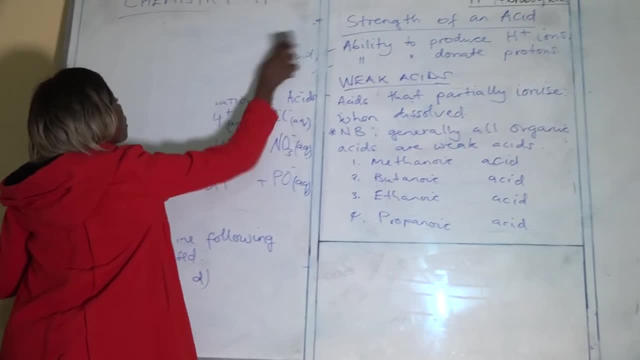 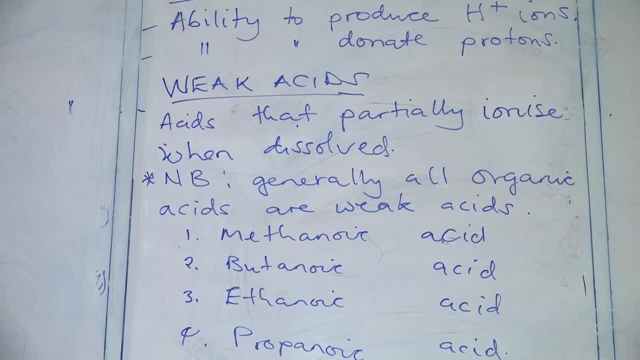 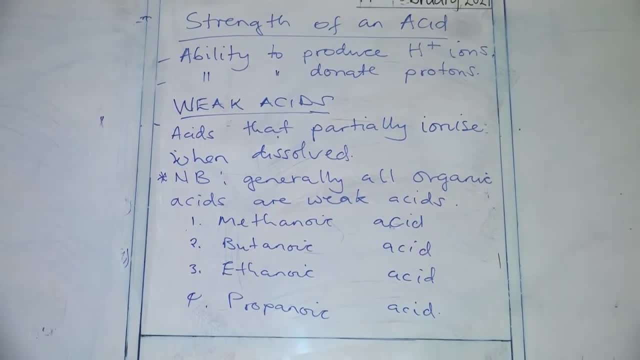 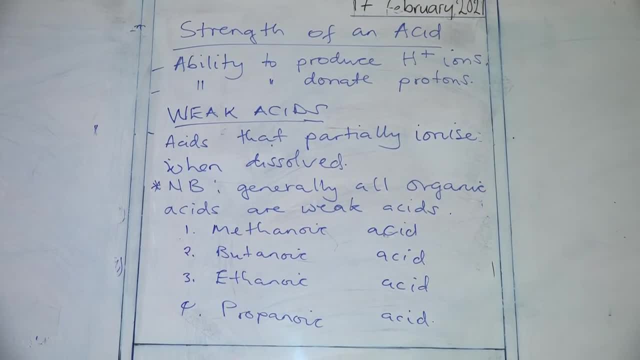 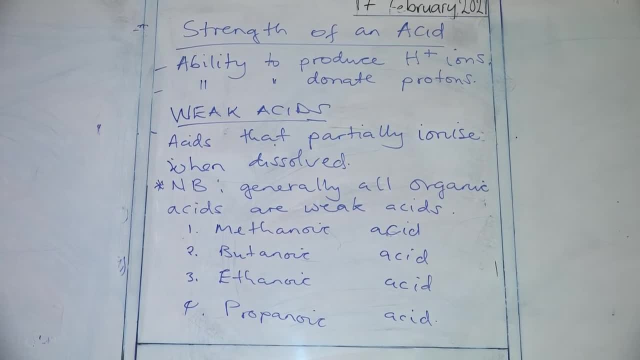 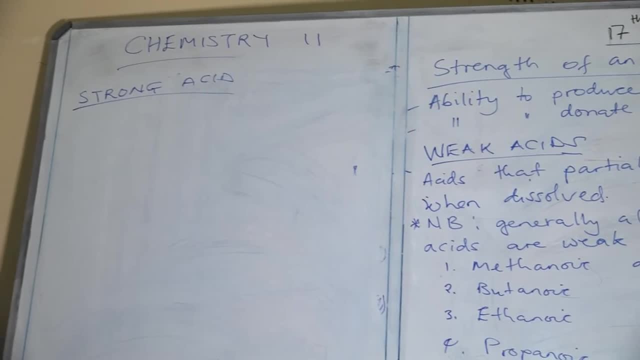 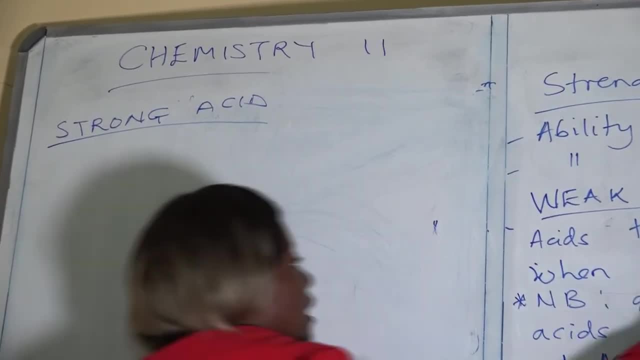 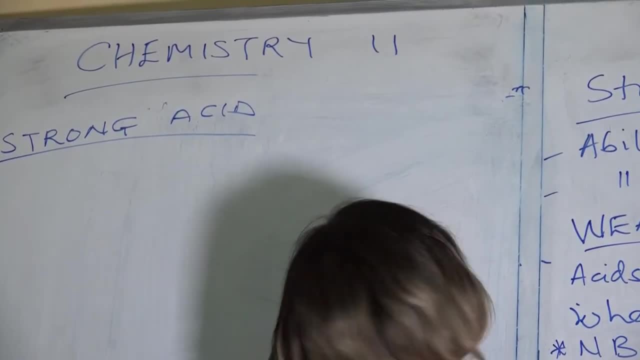 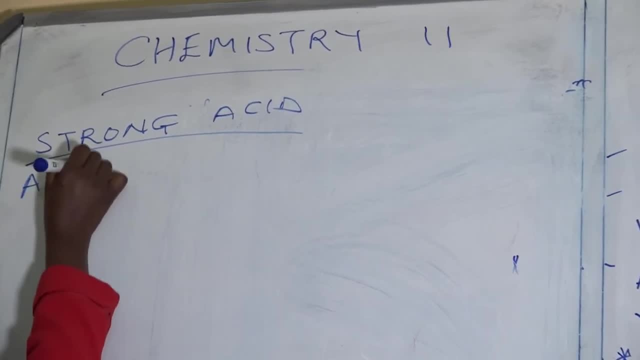 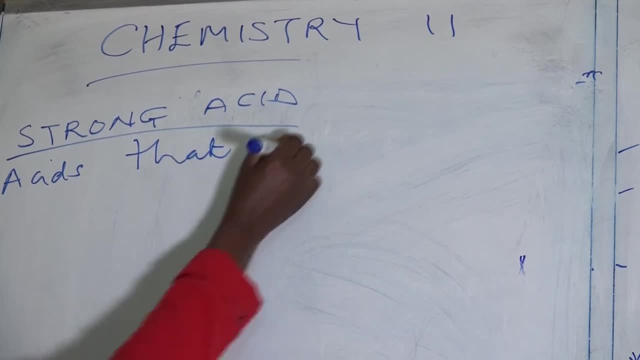 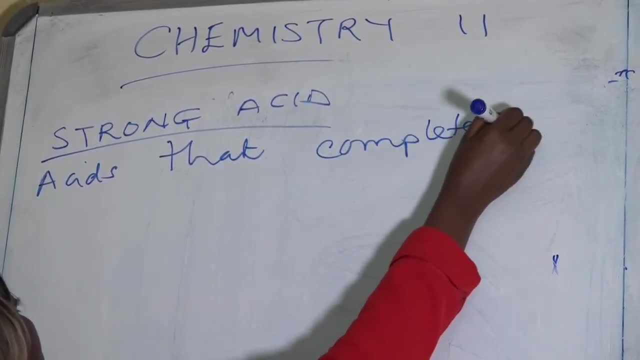 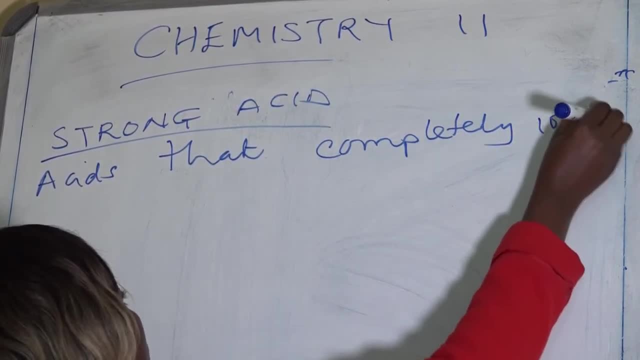 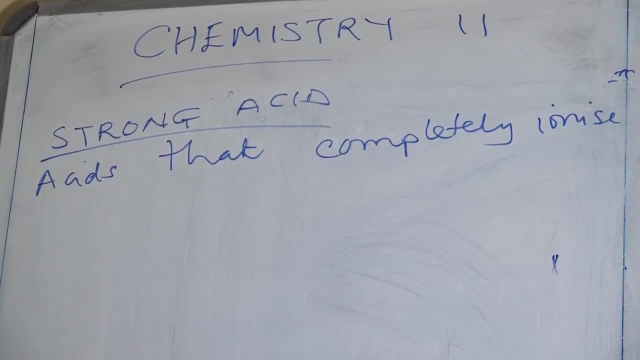 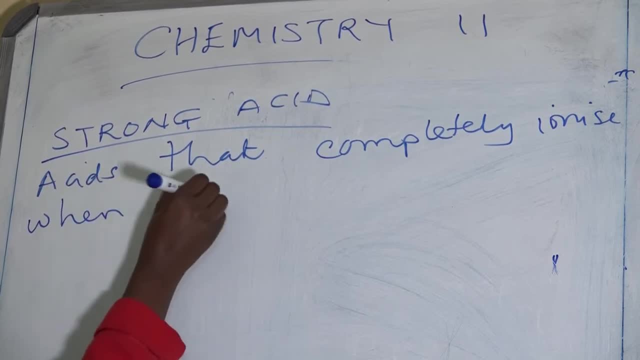 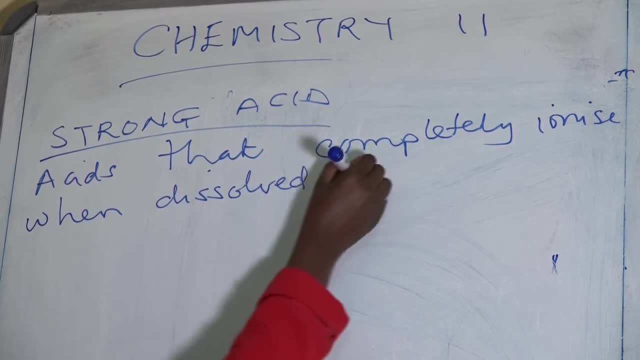 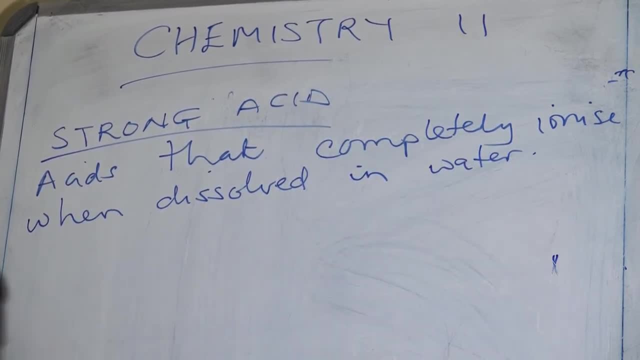 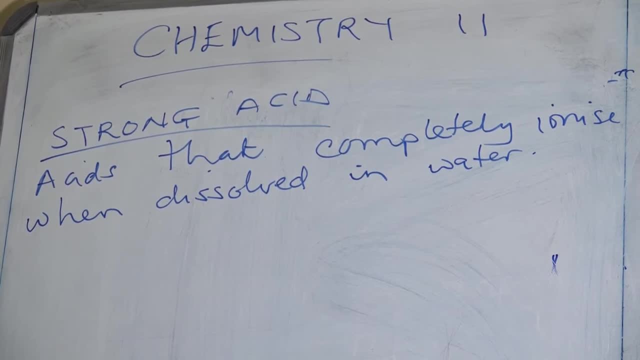 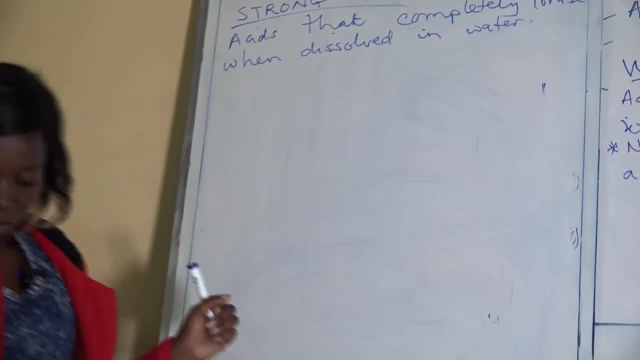 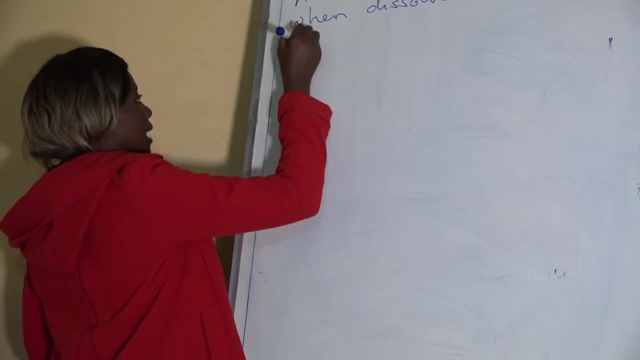 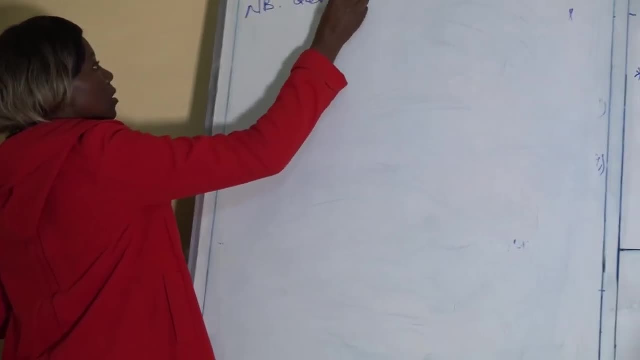 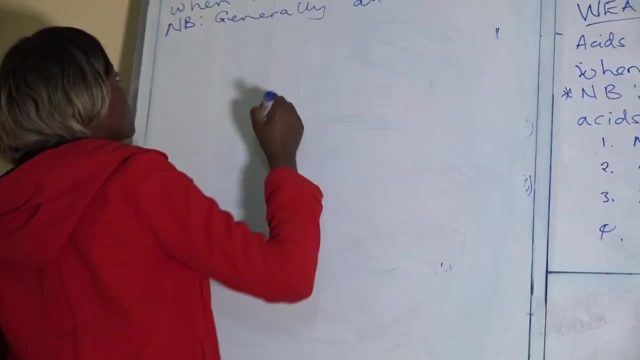 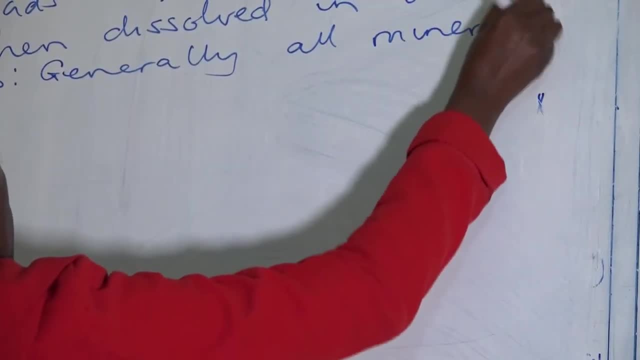 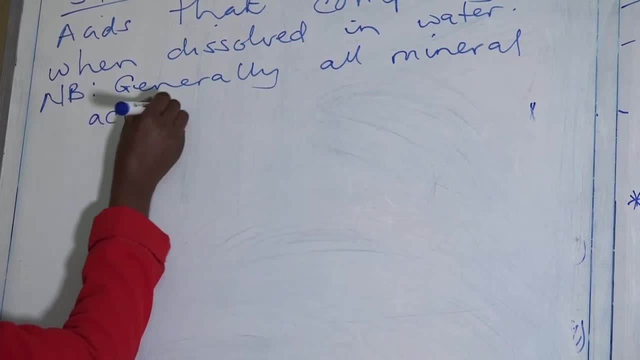 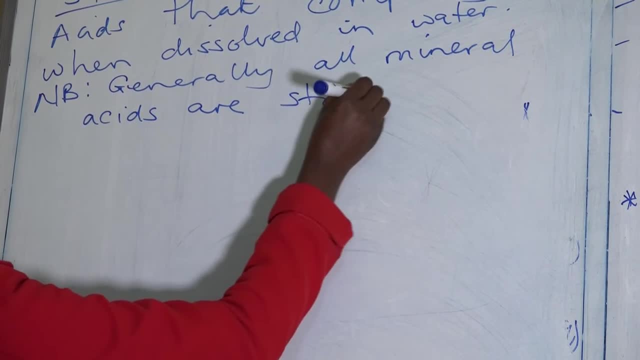 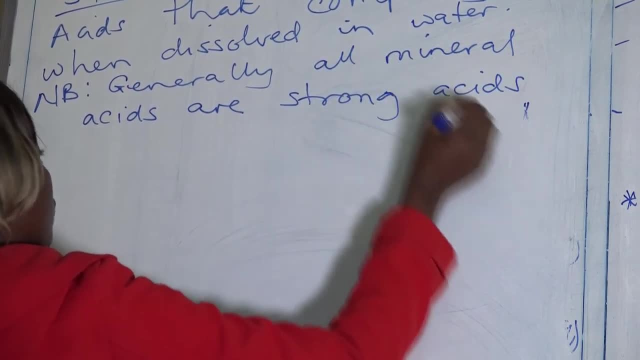 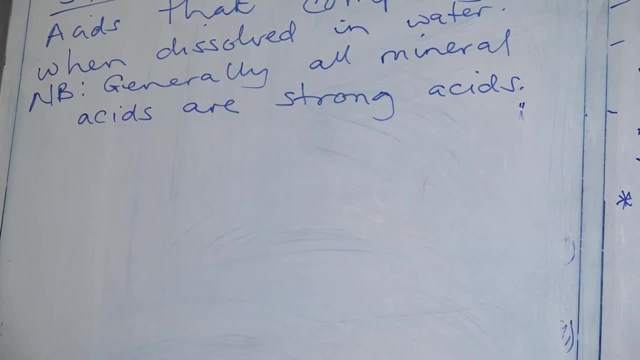 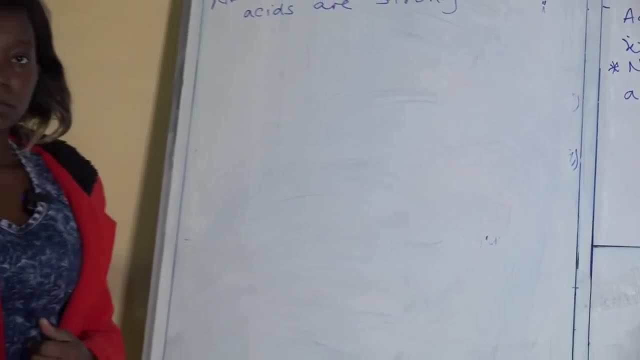 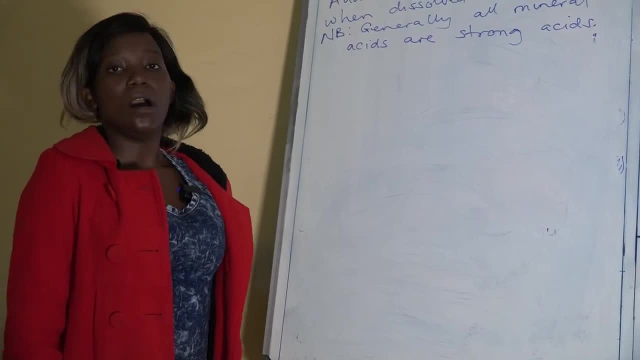 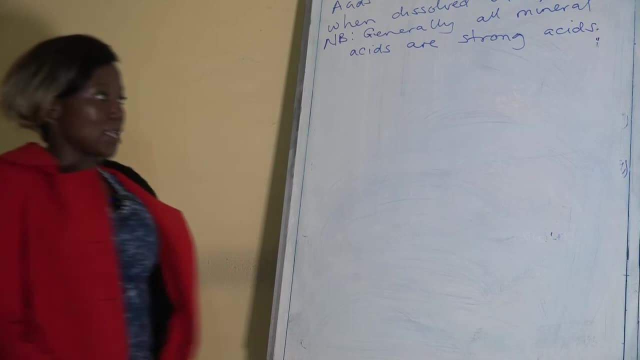 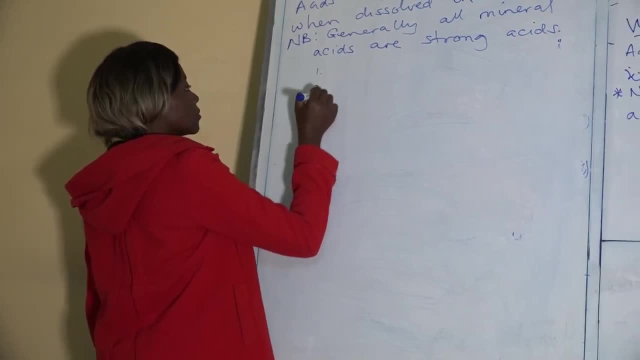 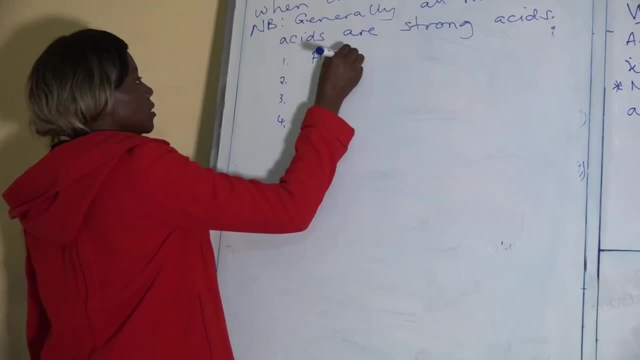 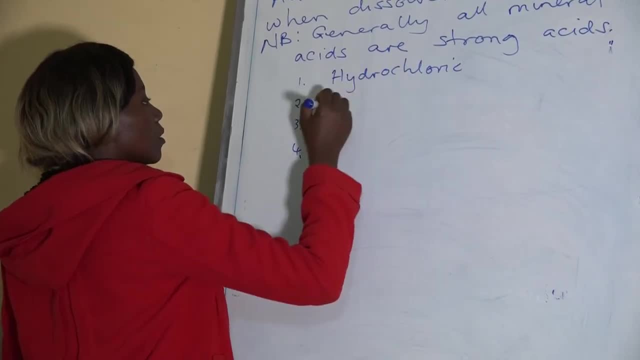 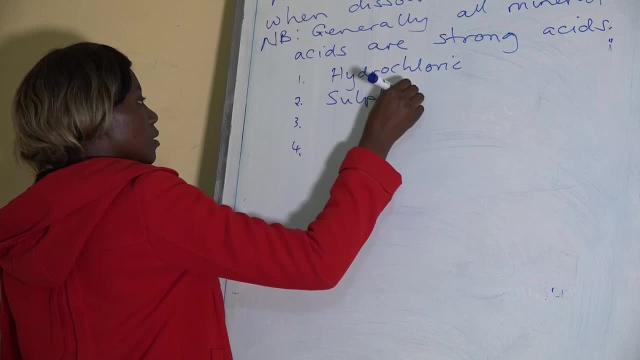 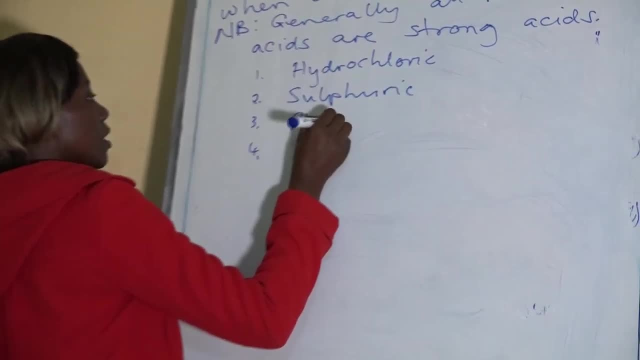 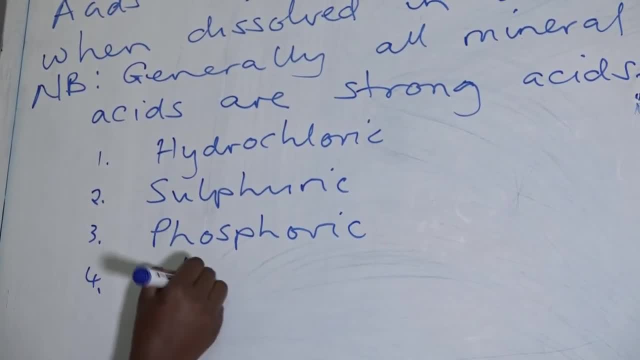 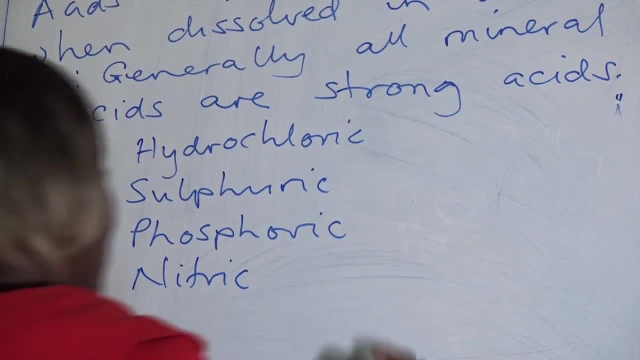 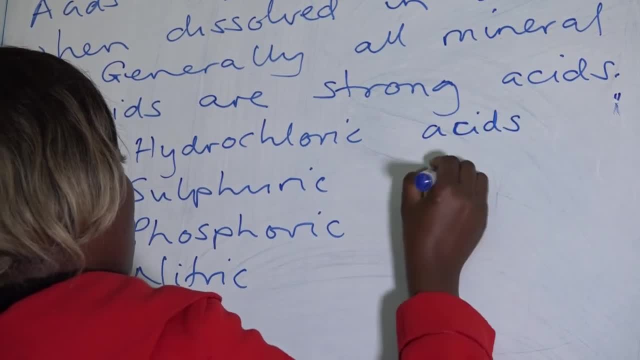 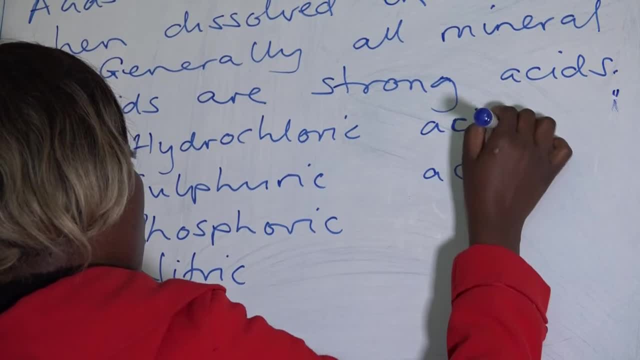 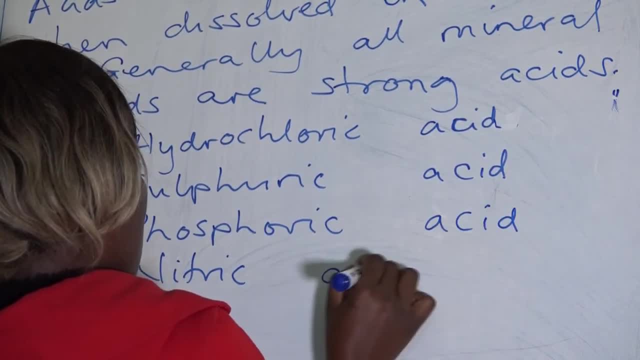 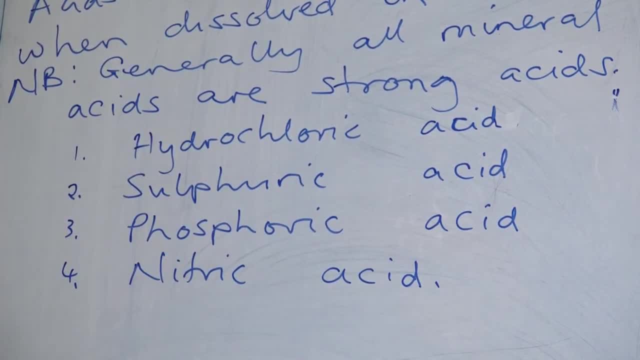 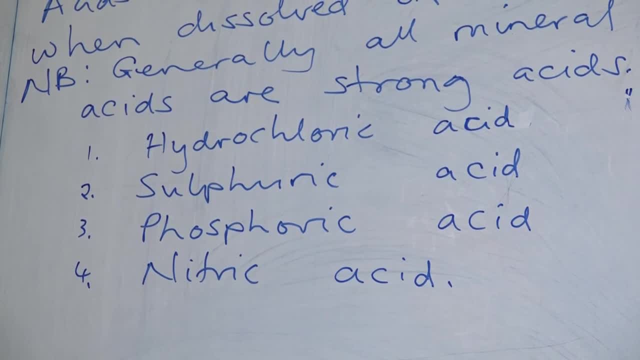 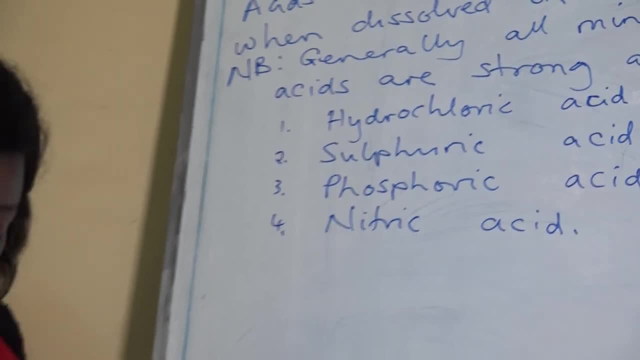 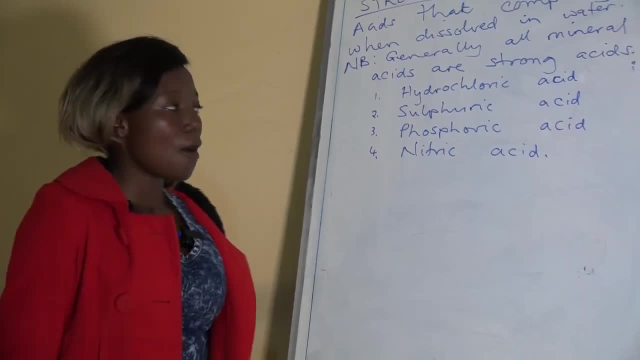 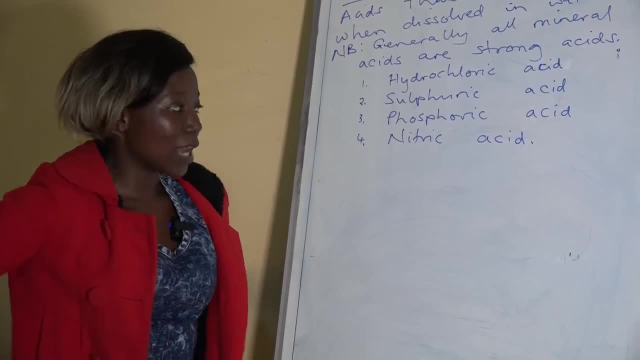 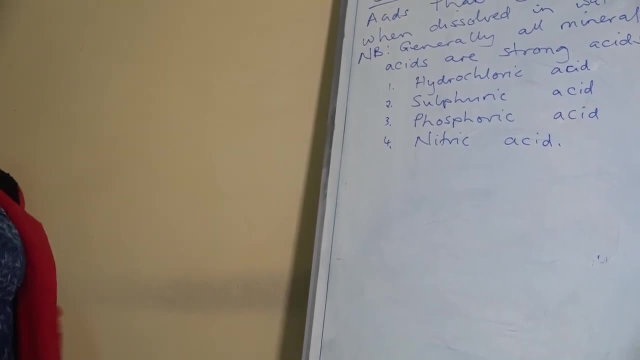 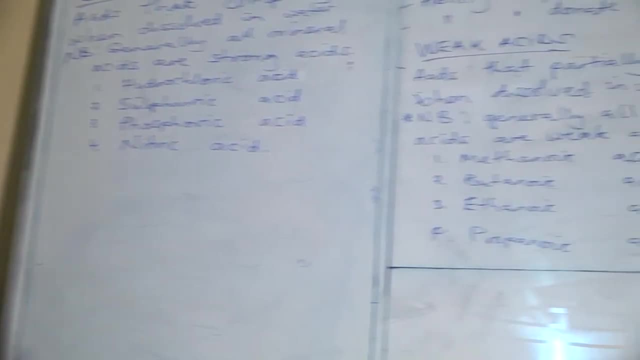 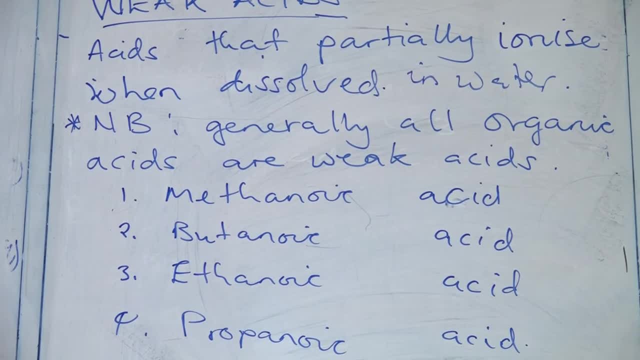 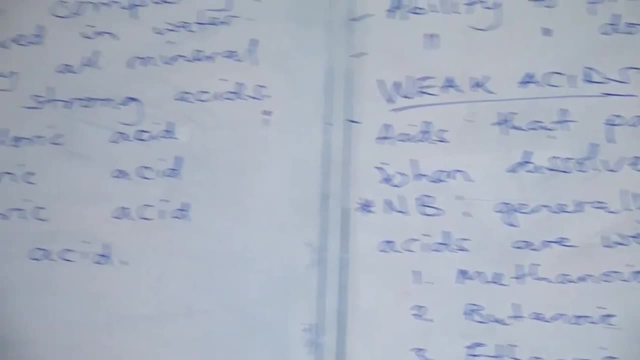 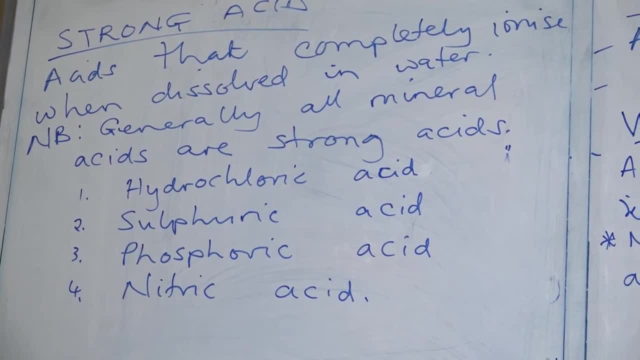 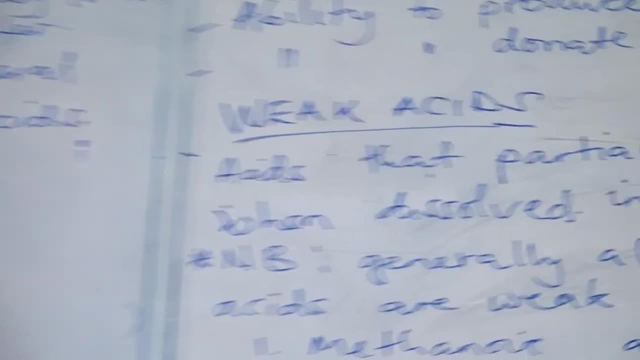 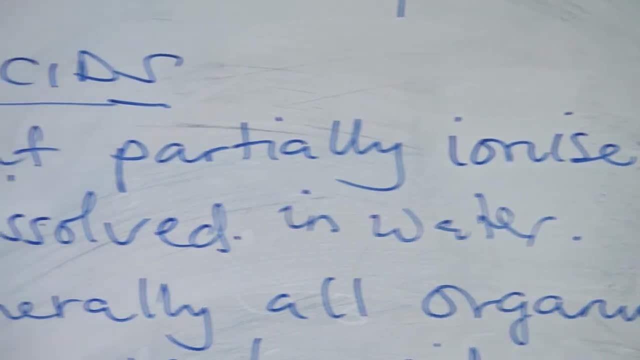 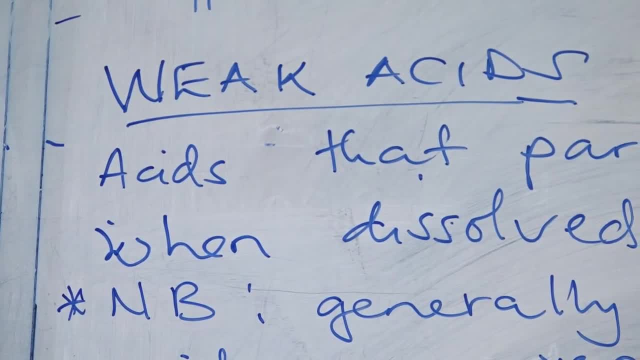 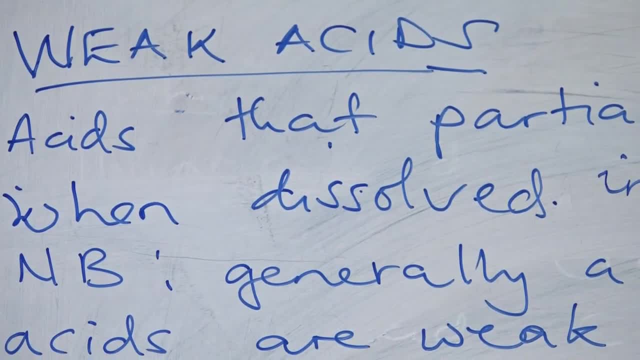 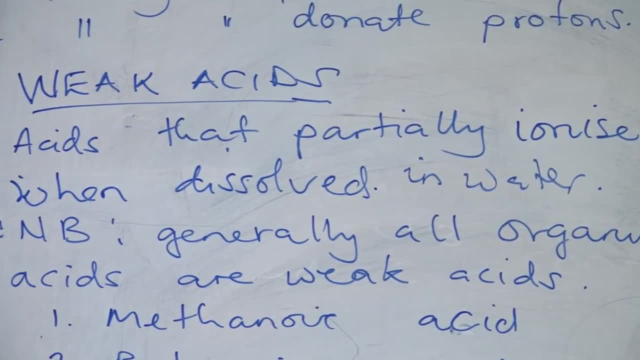